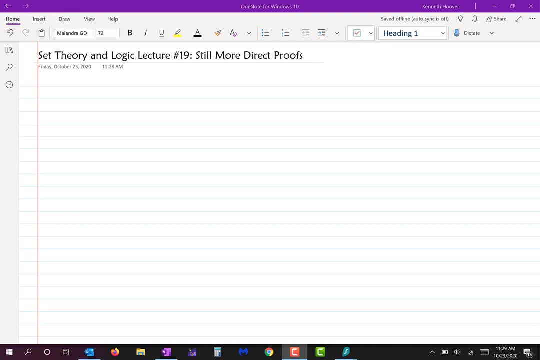 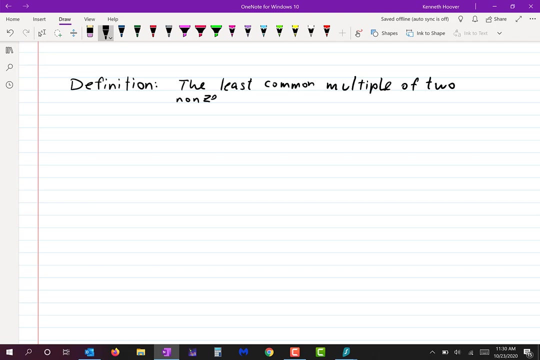 Okay, please look at this definition. This is the definition of the least common multiple of two numbers. The least common multiple of two non-zero integers of two numbers. The least common multiple of two non-zero integers of two numbers is the smallest number, the smallest natural number. 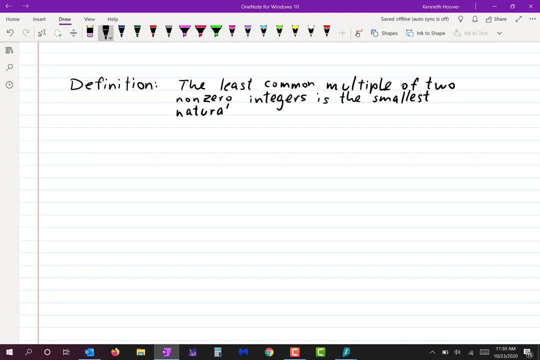 which means, by the way, implies that it's positive- The smallest natural number, that is, a multiple, multiple of both of them. okay, now we are going to prove this proposition. if a, B and C are natural numbers, then the least common multiple of CA and CB. 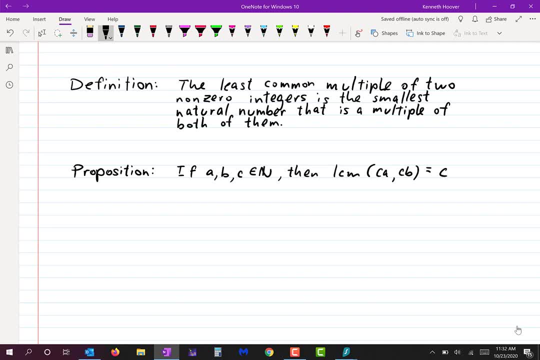 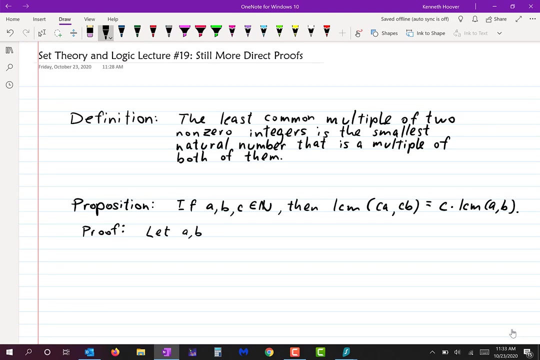 equals C times the least common multiple of a and B. okay, let's prove that. okay, so let's start with that: a, B and C be natural numbers. and here's what we're going to do. we want to prove that two things are natural, and one of them is that they are natural numbers. so let's. 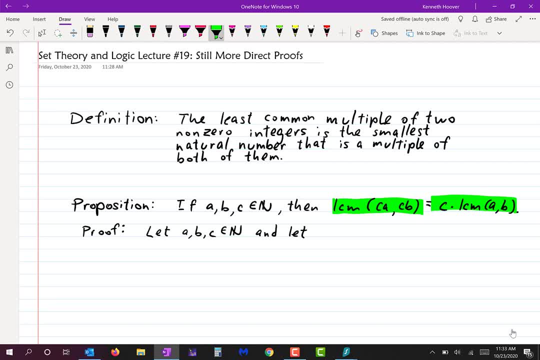 prove that two things are equal. one thing that we're going to do is just to save ourselves some time and writing. we're going to give them each a name, so let's call the first thing M and the second one at N. okay, so let M equal the. 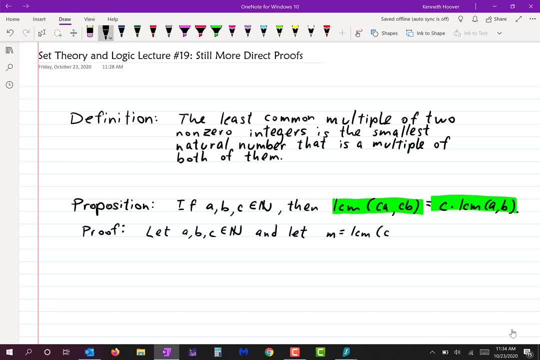 least common multiple of CA and CB and let N and equal to least common multiple of A and B. that is simply a convenience strategy, so that I can just write M and N instead of continually writing out LCM of ca and CB and C time, oh and um, LCM of A and B I meant to put. 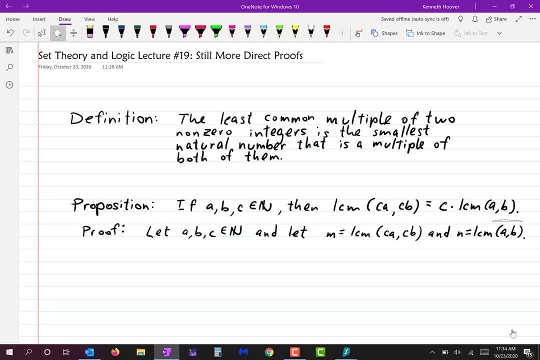 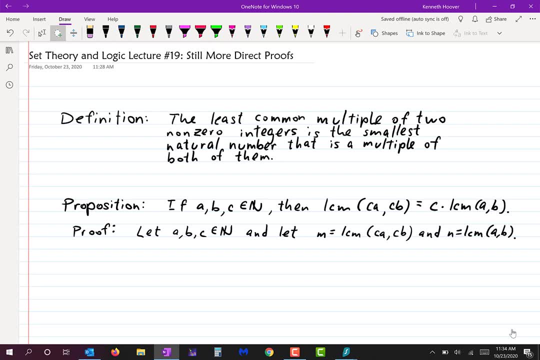 there though. sorry, I made a mistake. I meant to put c times, that to call that m, So let me shift that here. I'm just going to erase that. Okay, I meant to write c times, the least common multiple of a and b. 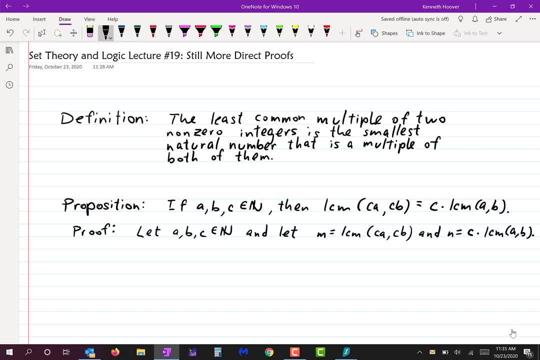 Okay, there we go. Okay, and what we want to do now is we want to show that m equals n. Now, here's a neat trick for that. Okay, you don't have to do it this way all the time, but oftentimes it is very convenient to try it this way When you want to show that m. 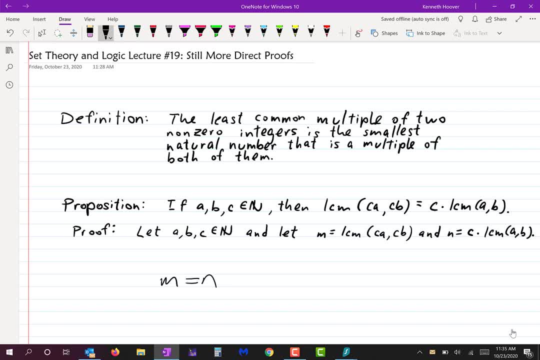 equals n. what you do is you show that m is less than or equal to n and n is less than or equal to m, or m is equal to or greater than n. Okay, if you can show that, then that means you have this. 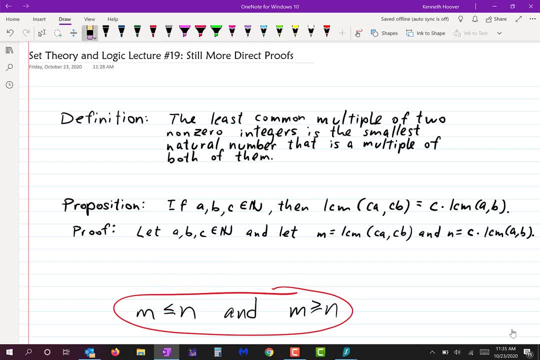 Okay, and that's the strategy that we're going to use. Okay, now, what do I know about the LCM of a and b? It is a multiple of a and it's also a multiple of b, right, And also it's a natural number. Okay, that's just by the definition of least common multiple. 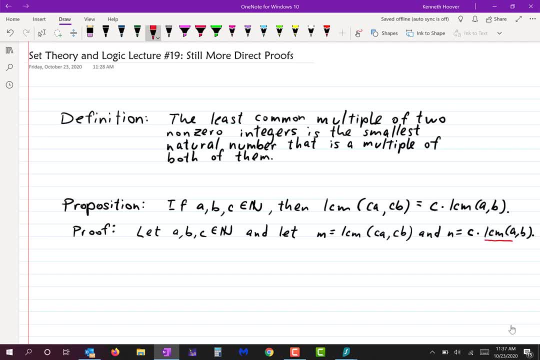 So look at this thing, Not n, but just this part: LCM of a and b. I know that it is the smallest natural number, That is, a multiple of a and also a multiple of b. Okay, so I can say then: 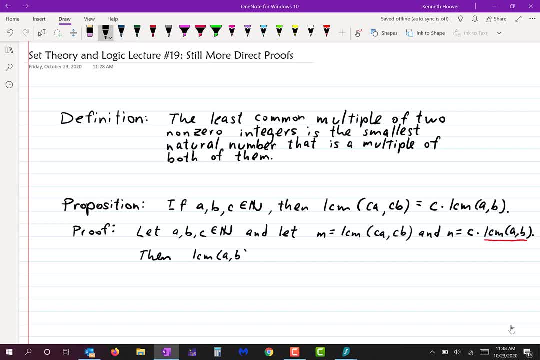 the LCM of a and b is a multiple of a and b, So it equals a times x for some. Now just follow along here. I'm going to write some stuff out, but then I'm going to show you how I can save some time. Okay, so the LCM of a- b equals a times x. for some x, That is a natural. 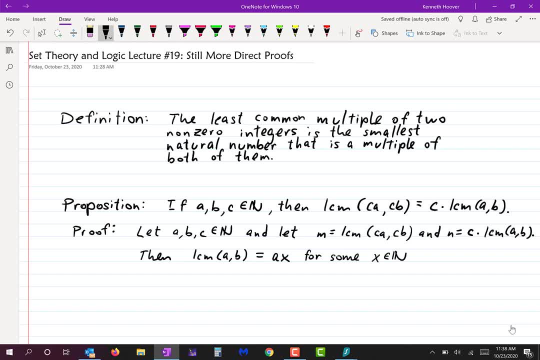 number, Okay. and also I can say that the LCM of a and b equals b times y. for some natural number, y, Okay. and I could then say: hence ax equals by Why? Because they're both equal to the LCM of a and b, so they're equal to each other. 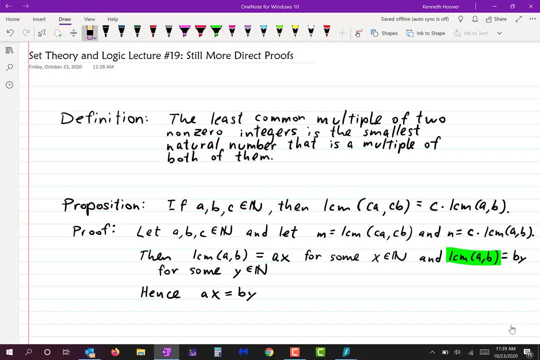 Now I can say all of that in a shorter fashion. Watch, I could say: the LCM of a and b equals ax and also equals by for some x and y. that are natural numbers. And why is that? That is by the definition of least common multiple. Okay, 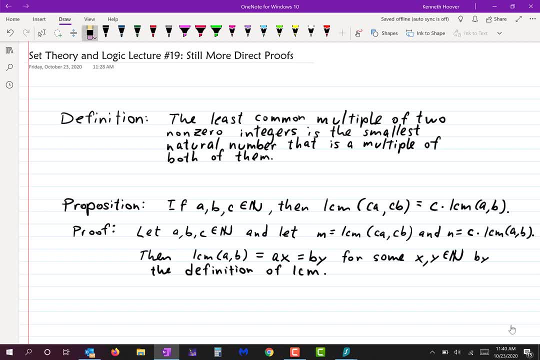 I'm just going to throw this out here. I haven't said it yet, so I'll say it here: My LCM of a and b equals a times x. I'm going to start with. the LCM of a and b equals b. Why? 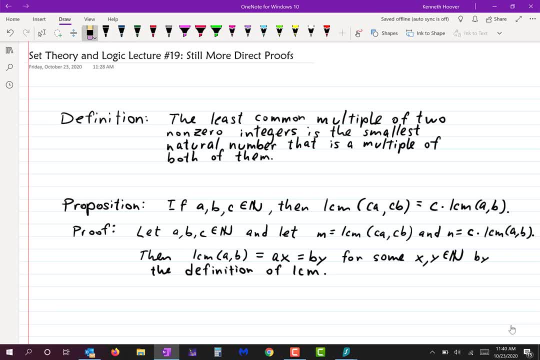 The reasoning that you're giving to justify your logic doesn't have to be said at the end of the sentence. We could certainly do this. I could certainly have said by the definition of LCM: the LCM of A and B equals A times X and also B times Y. 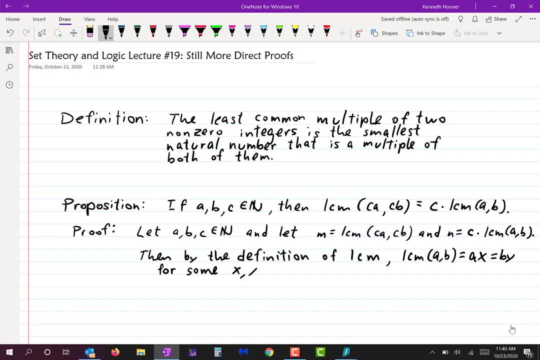 for some natural numbers: X and Y. Sometimes we put the reasoning at the end, sometimes at the beginning. You just change it up a little bit so that things don't get boring. I could also have done this, by the way. I could have said that X and Y are natural numbers before I said. 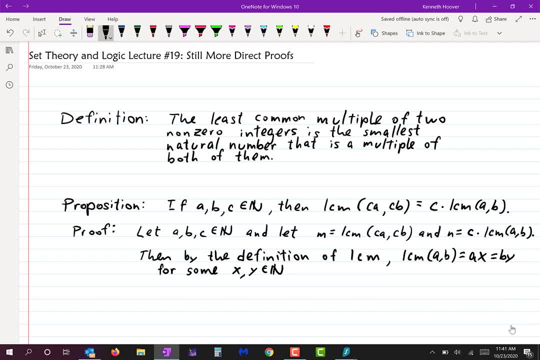 that the LCM of AB equals AX, and BY What I mean is this: I could have said that by the definition of LCM there exist natural numbers, X and Y, such that I think it's okay with me if you just want to put ST. 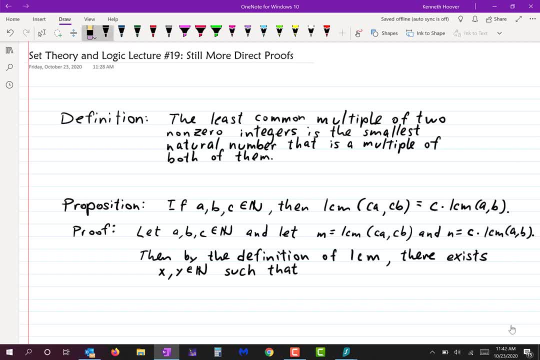 for such that時指肥米. Okay, such that is okay with me. It's just okay to put St for such that, because ST is important for me. in this case, the LCM of A and B equals AX, which is also equal to BY. okay, now let me just 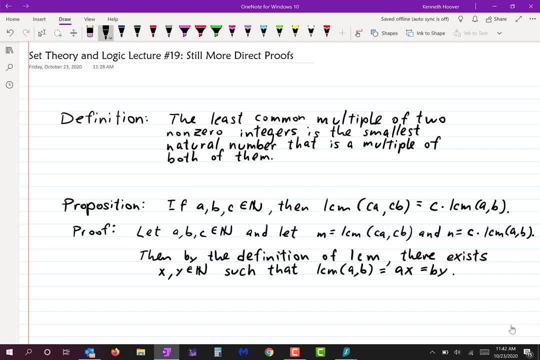 one more thing I want to say about this line here. another option, one more option. so I have just a small bone to pick with this: the way it's written. we read in our culture from left to right. so when I read that, this is what I'm thinking, I'm 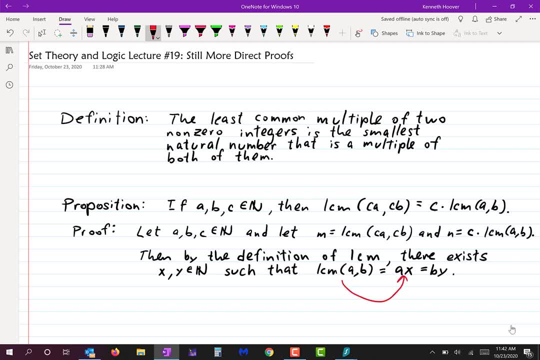 thinking you have the LCM of AB equals AX and AX equals BY. okay, why do I know AX equals BY? because they're both equal to the LCM of AB. so personally, I think it's slightly better. I think this is maybe a little bit confusing. it looks. 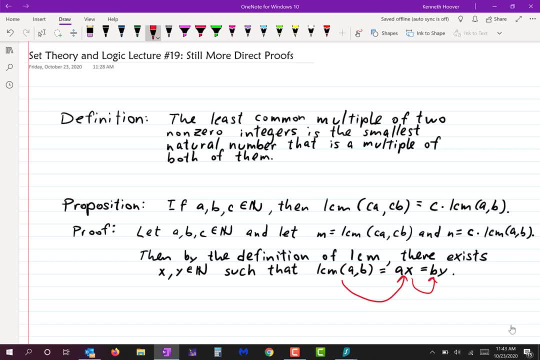 it looks. When I look at this way this is written, it looks to me like AX is linked to the LCM of AB and BY is linked to AX, When the reality is they are both equal to the LCM of AB and that's why they're equal to each other. I personally think this would be a little bit better. 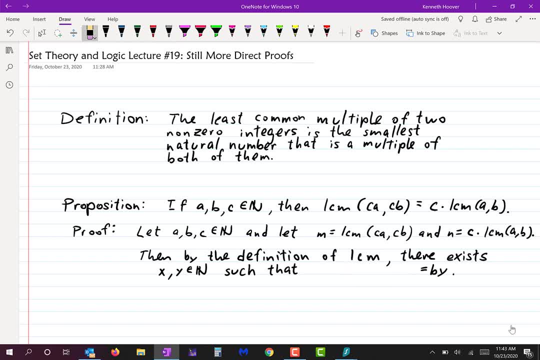 written like something like this. I didn't really change anything mathematically, but personally I think that's a little bit more straightforward. It says AX equals the LCM of AB and BY equals the LCM of AB. OK, and because of that, AX will equal BY. I think that's a little bit better. 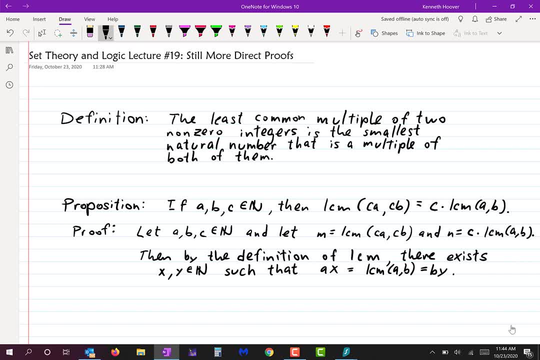 OK. So what does that tell us about N? Remember, N is C times this, Right? So wouldn't that mean that C times A times X would equal N, And also C times B times Y equals N, And therefore C times A times X equals C times B times Y, Correct? Do you agree with that? 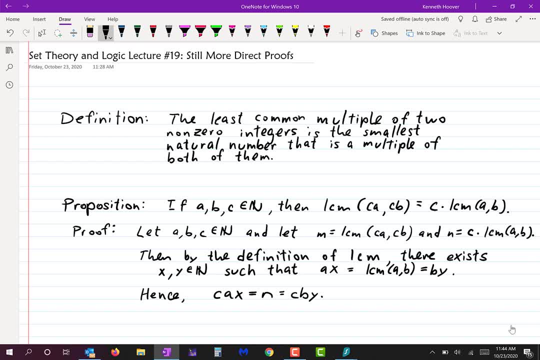 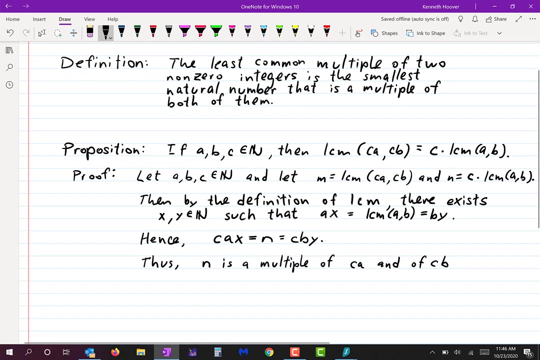 So doesn't that show that N is actually a multiple C, A and also a multiple of C, B, Subtract 2.. Subtract 3. And она является с разама c результат and of cv, Correct, Okay? Also, what kind of number is n? What group of numbers does it belong to? It's a natural number, right? How do I know n is a natural number? 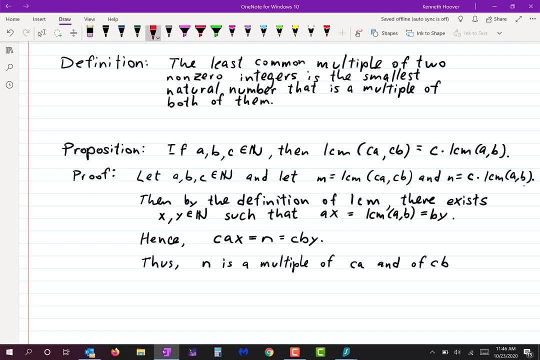 Because, by definition, the LCM of a and b is a natural number And we are given that c is a natural number and a natural number times a natural number is a natural number, So let's point that out. Also, n is a natural number. 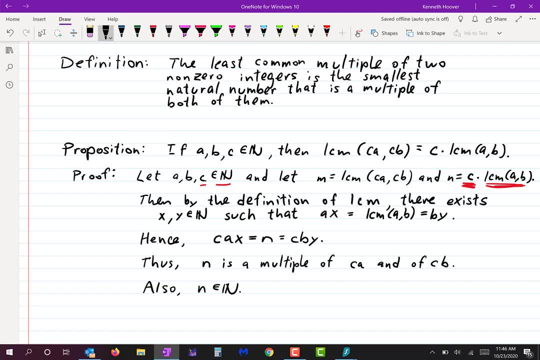 Okay, Why did I not write down reasonings for the last three lines? Because it was just basic algebra type stuff. That's why- Let's look What was my reasoning for this line right here. All I did was substitution right. I already had up above ax equals by 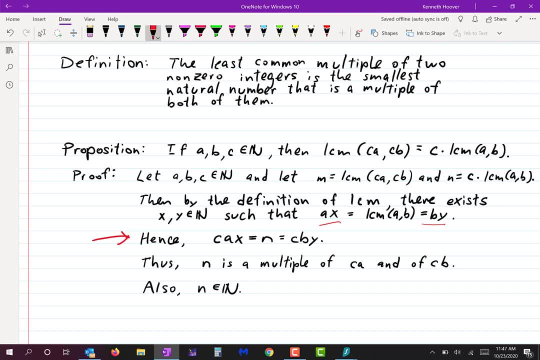 And so, therefore, by the multiplication property of equality, c times ax equals c. And so therefore, by the multiplication property of equality, c times ax equals c, c times ax equals c, c times by right And by substitution: c times ax equals c times the LCM of a and b. 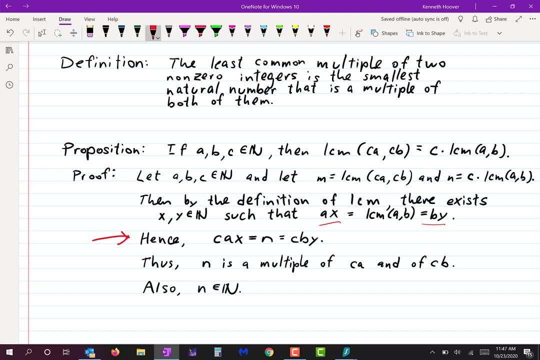 which is what we decided to call n. Okay, So I wasn't using any rules of inference or anything like that, I was just using substitution. I was just using substitution and multiplying both sides of an equation by c. Okay, What was my reasoning for this? 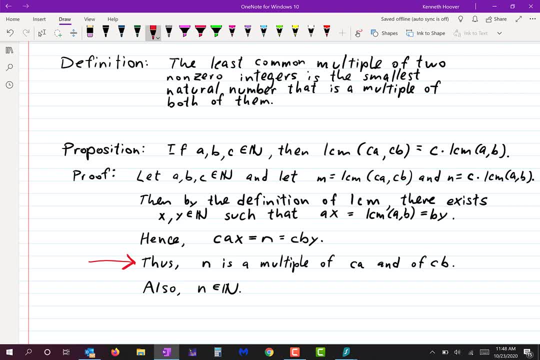 I didn't write a reasoning down, but what was it? That's just the definition of multiple. You can write that if you want. I'm a little on the fence on that one. Is that something that's important enough to write down? 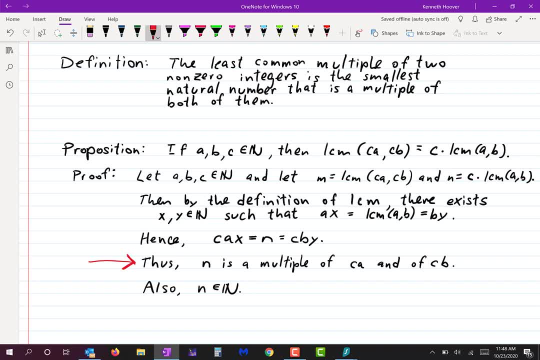 Not just important, but remember what I said before. For a reasonable person would I need to give that reasoning? How do I know n is a multiple of c a and c b? How do I know n is a multiple of c a and c b? 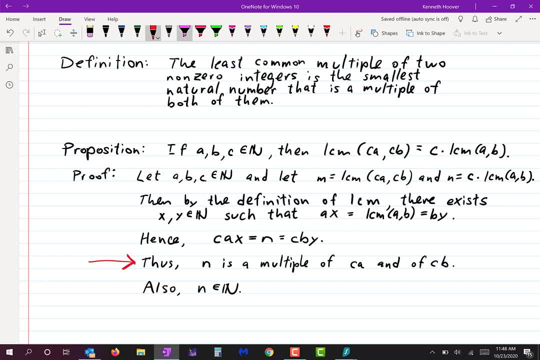 I don't think that that's necessary. It's right here. Look, n equals a multiple of c a And it also equals a multiple of c b. I would certainly not discourage you if you wanted to write. I would certainly not discourage you if you wanted to write. 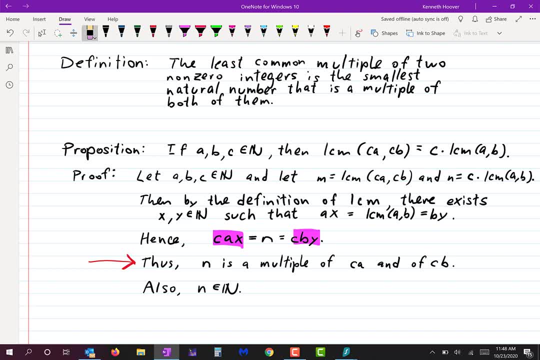 I would certainly not discourage you if you wanted to write just a second here, if you wanted to write by the definition of multiple, Okay, But I don't think it's absolutely necessary to write that. But I don't think it's absolutely necessary to write that. 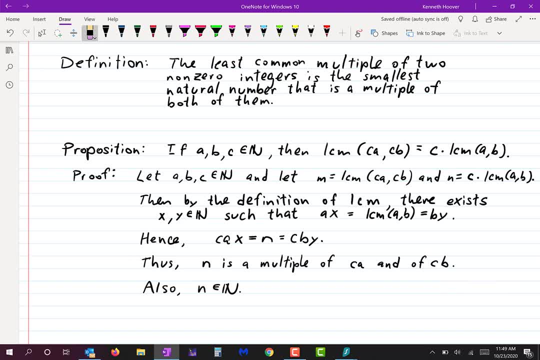 That's why I didn't. I think being a multiple of something is a pretty trivial concept and I wouldn't expect somebody would need me to point that out to them. Okay And last question: How do I know n is a natural number? 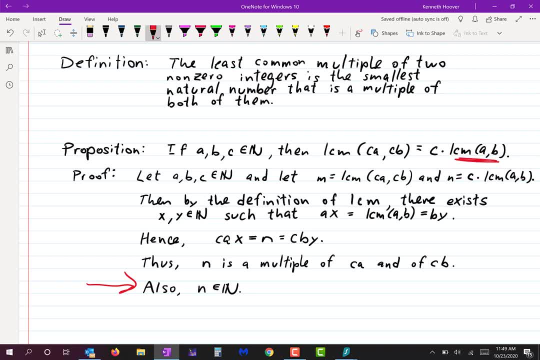 Well, because I said earlier, because we know this is a natural number. We know this is a natural number. Oh sorry, I actually meant to underline those here. We know that's a natural number. We know that's a natural number. 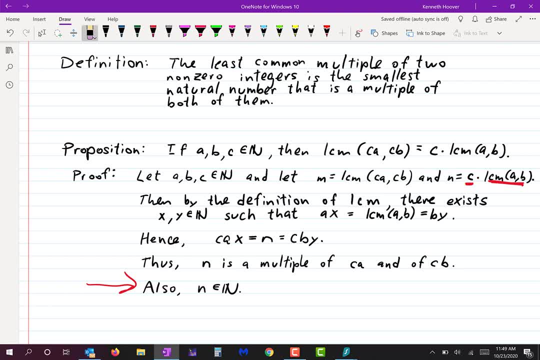 And we know that two natural numbers multiplied together give us a natural number. I've already mentioned several times that I mean that's technically called the closure of the natural numbers under multiplication, but I don't think that is necessary to write that down every time you use it. 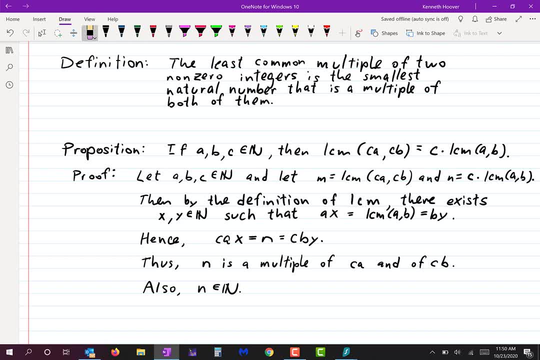 Maybe if it's not obvious in you know one instance, then you would maybe want to write it down. Okay, So I could do this. If I think that that's not obvious- why n is a natural number, I could do this. 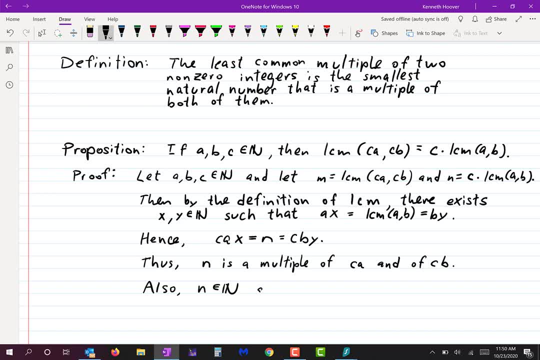 I could say also: n is a natural number, since c is a natural number and the LCM of a is a natural number. Okay, LCM of a and b is a natural number Then, since n is just the product of those two things. 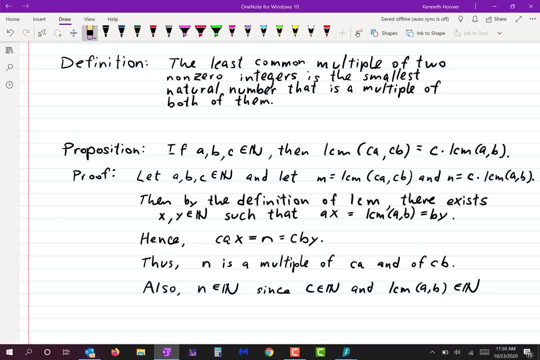 that's why n is a natural number. Okay, All right, Now let's move forward. So n is a natural number and it's a multiple of ca and it's a multiple of cb. So what do I know about the relationship between n and m? 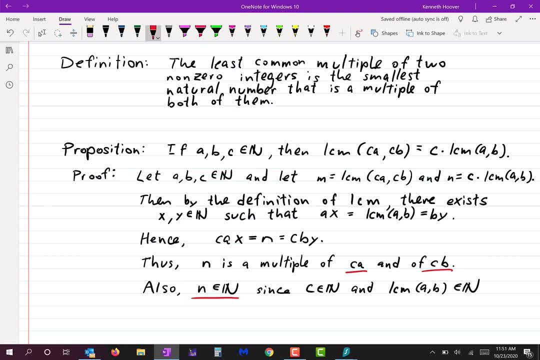 Think about that Well. m is the least common multiple of ca and cb. right n is a multiple of ca and cb and that means that n is a common multiple of ca and cb. m is the least common multiple of ca and cb. 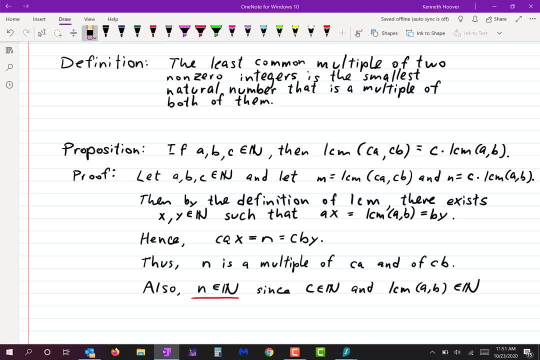 So what's the relationship between m and n? Doesn't that mean that m will be less than or equal to n? Because n is a common multiple of ca and cb and m is the least common multiple of ca and cb, and so therefore m cannot be greater than n, right? 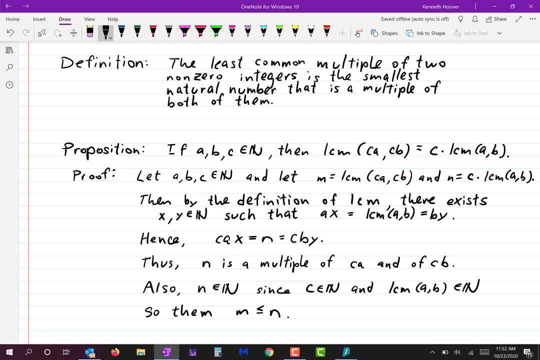 Do you see that reasoning there? Okay, and now we're going to do basically the same idea with m, showing that n can't be bigger than m. Okay, so we're going to do this. We're sort of switching to the other side of the coin. 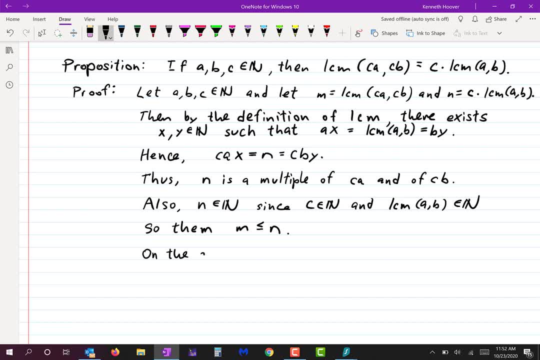 So I like to use the phrase on the other hand to tell the reader: okay, I'm switching to a different line of thought now. Okay, so don't think. to the reader I'm saying, don't think that what I'm about to write is because of this. 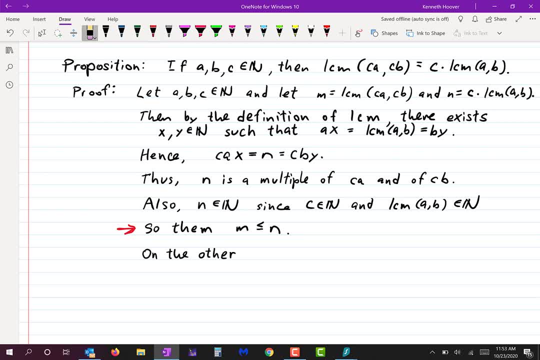 It's not Just leave that line, just leave this line on the back burner for a minute. and now I'm going to start a new thought. Okay, On the other hand, okay, and now we're going to look at the number m. 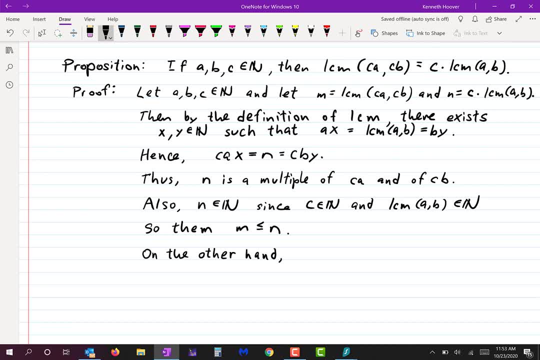 Okay, I'm going to say, by definition of LCM, there exist two natural numbers. What would you like to call them? I won't call them x and y. I've already used that for something and I don't want to cause any confusion. 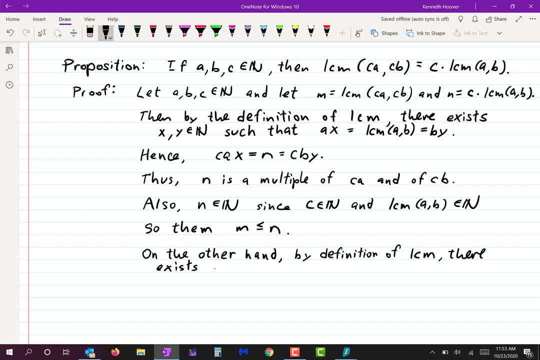 So what should we call them? How about j and k? There exist natural numbers, j and k, such that, what? Such that c a times j equals the LCM of c, a and c b. Let me go ahead and write that down. 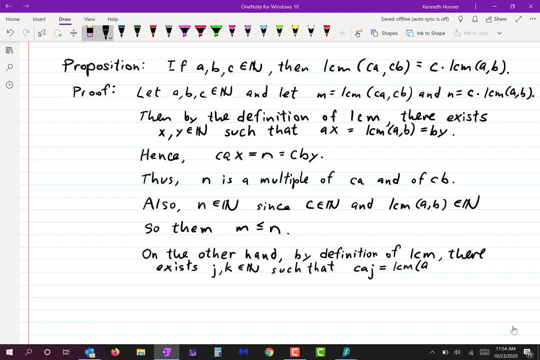 but I'm going to change that in a second. You'll see why. Whoops, I forgot to write the c, Okay, and also c b times k equals the LCM of c a and c b, Okay. so I just want to point out to you. 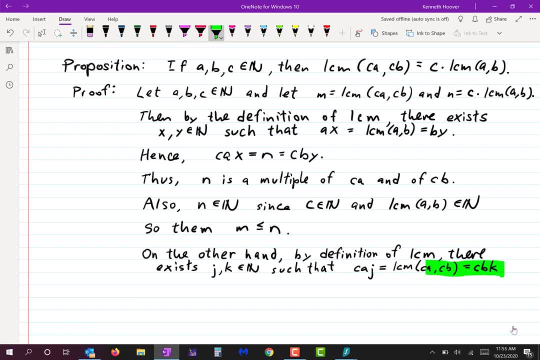 what I'm doing here is essentially the same thing I had done there. Up above, we were looking at the LCM of a and b. Down here I'm looking at the LCM of c a and c b. Okay, But I'm doing the same idea. 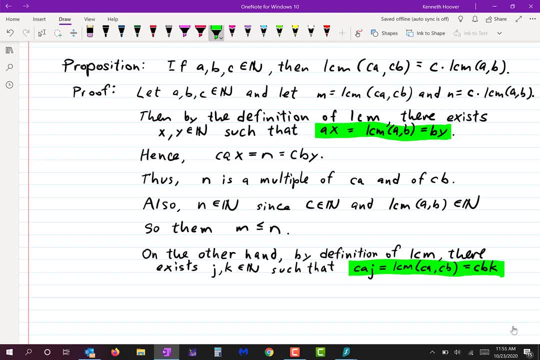 And the only other thing I want to change is that up above this, right here, was not exactly n, n is c times that. Down here, though this thing right there, is exactly m, So let's save some space there. 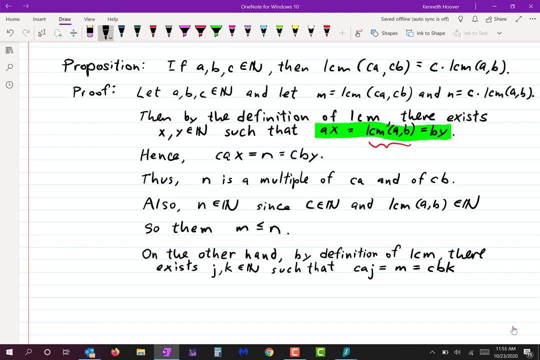 and just put m. Okay, Alright, Thus, m is a multiple of what? What do you think? It's a multiple of a and b, Right? Do you agree? Because why? Let's look at this: m equals c, a, j, right? 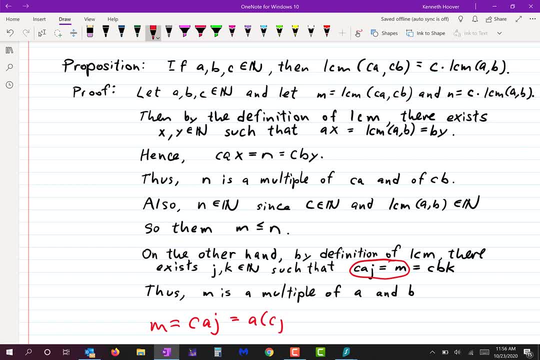 And isn't that the same thing as a times c j Right Using? what properties did I just use there? Just the commutative and associative properties. Okay, If you feel like you want to point that out, that's fine. You can always do this right up here. 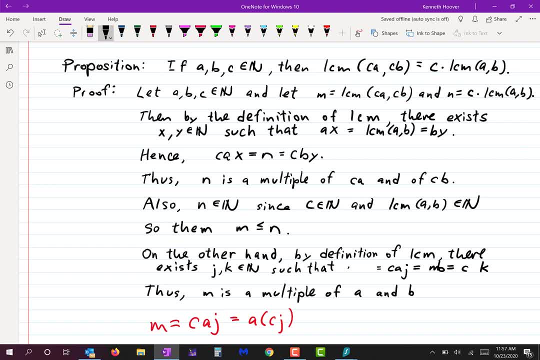 I could actually have written: a times c: j equals c. times a: j, which equals m, which equals c, times b. times k, which equals whoops, b times c, k. Right, I could have written that, And now it's totally clear that m is a multiple of a and b. 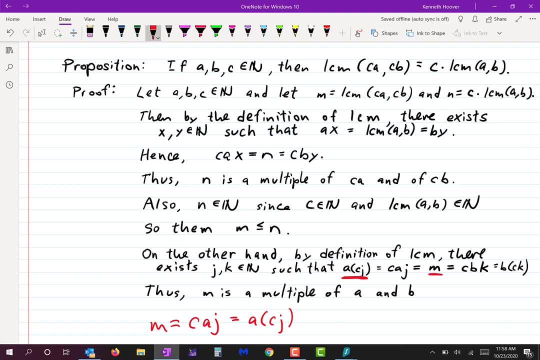 because m equals a times the number c- j, and m equals b times the number c- k. So m is a multiple of a. m is also a multiple of b. And what kind of number is m? m is a natural number. Why is that? 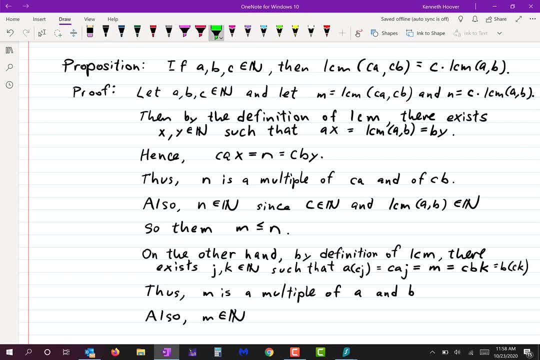 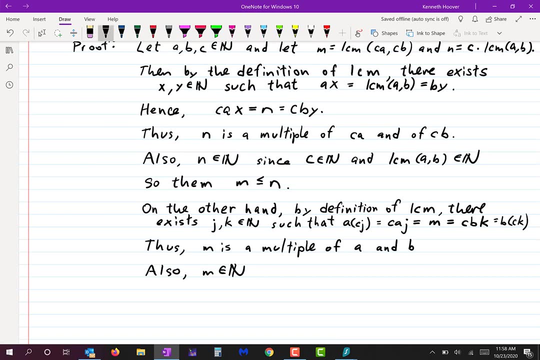 Because m is the least common multiple of two things, And in the definition of least common multiple it says that such a number is natural. So n, since m is a common multiple of a and b, and n is the least common multiple of a and b. 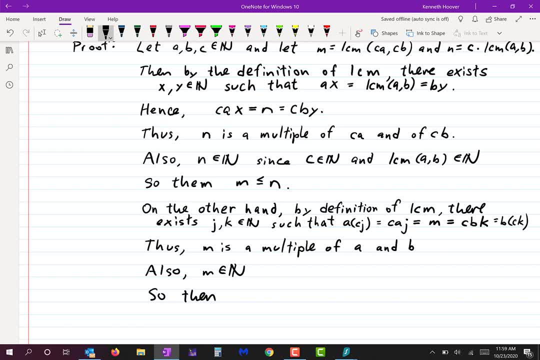 then n cannot be bigger than m, in which case n must be less than or equal to m, And then we can say: therefore, m equals n. But I want to add to this: Okay, why? Why does m equal n? 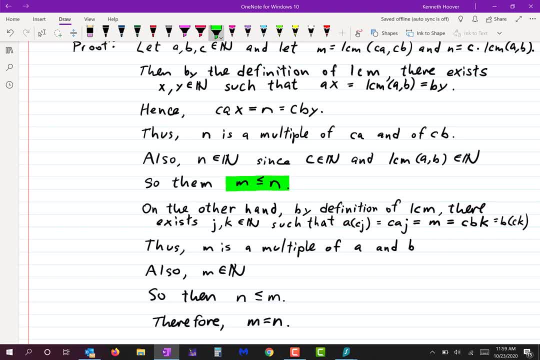 Because here we showed that m is less than or equal to n, and here we showed that n is less than or equal to m. So I think I should just point that out, that that's the reasoning I'm using to get this Okay. so let's add that reasoning in. 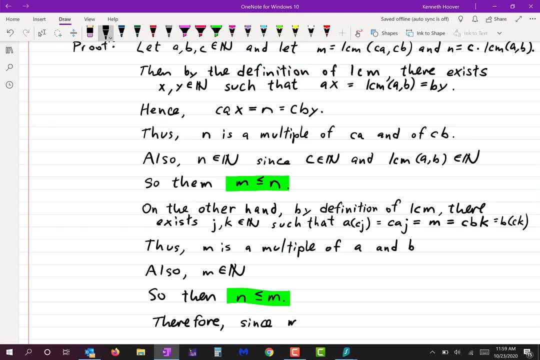 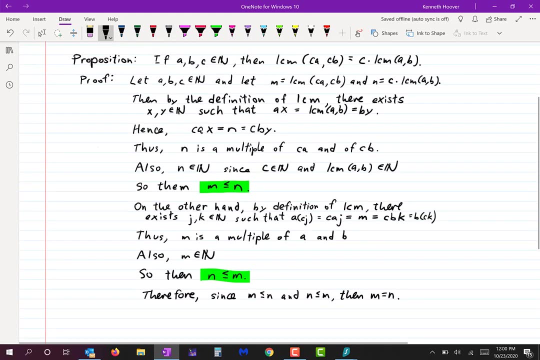 Since m is less than or equal to n and n is less than or equal to m, then m equals n, And that's what we were trying to prove, Because that's m and that's n, and we were trying to prove that they equal each other. 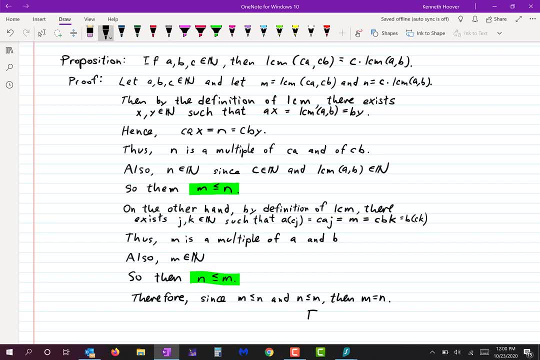 So that's what we did. That means we're done. Okay. and one other thing Again. this is just a matter of word choice. This is not logic, and so it doesn't matter if you do this or not. It's just up to you. 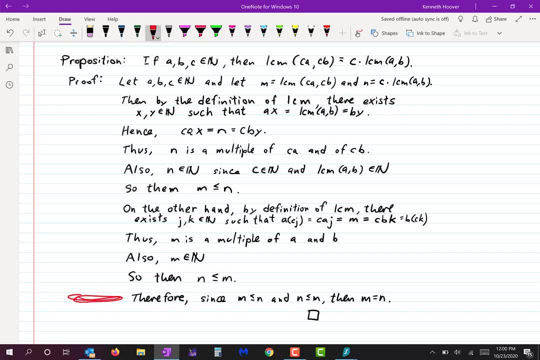 Is that because the reasoning of this came from two very separate things. I like myself to put the word finally there instead of the word. therefore, That's just personal preference. So let me explain again why I think that. Because there's three. 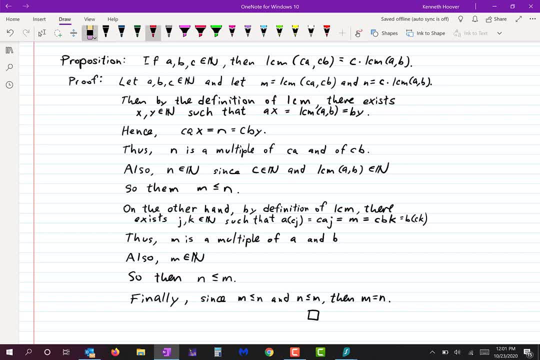 there's three parts to this proof. Part one was this And part two was something totally different. This, They're unrelated to each other. And then, finally, part three is to put the first two parts together, And that's why I like the word finally there. 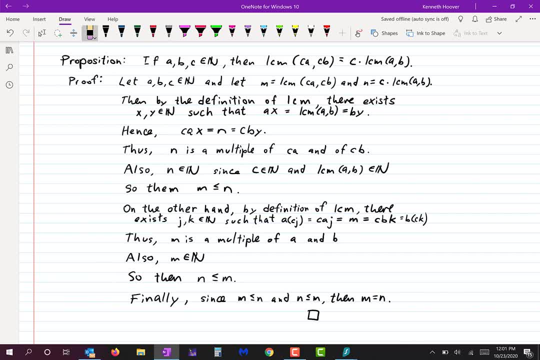 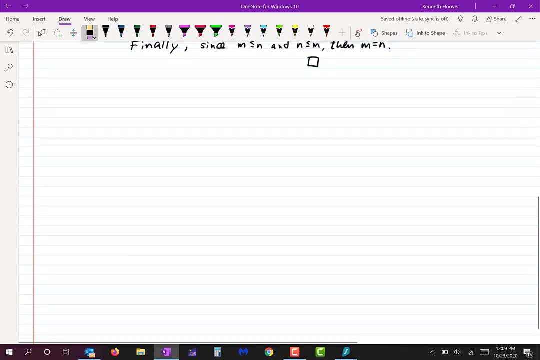 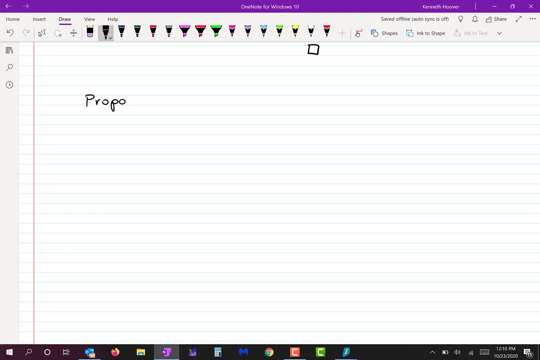 Okay, Alright, So that's the end of that proof. That was a bit longer than the other ones that we've practiced. Okay, Next proposition we're going to prove. This one's going to be short. Let x and y be positive. 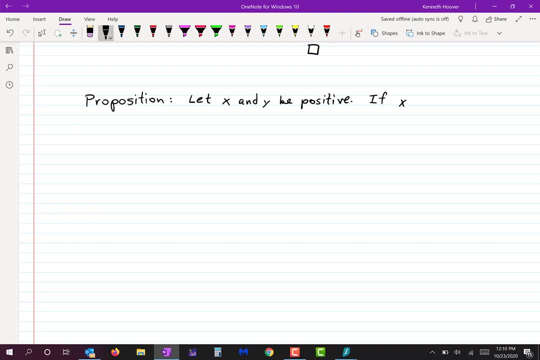 If x is less than or equal to y, Then the square root of x is going to be less than or equal to the square root of y. Okay, Let's prove that. So let's put down our given So: 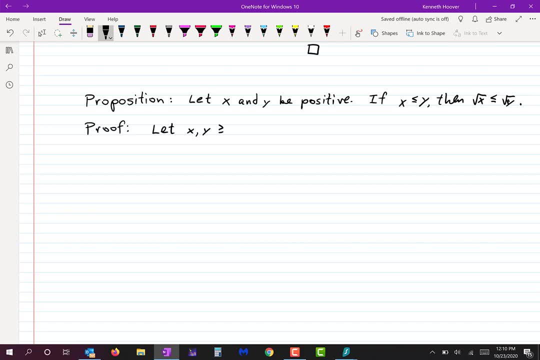 let x and y be positive. Oops, I'm going to write it like that. It's quicker than writing out the word. Okay, And what else do we have there? It says: if x is less than or equal to y, then blank. 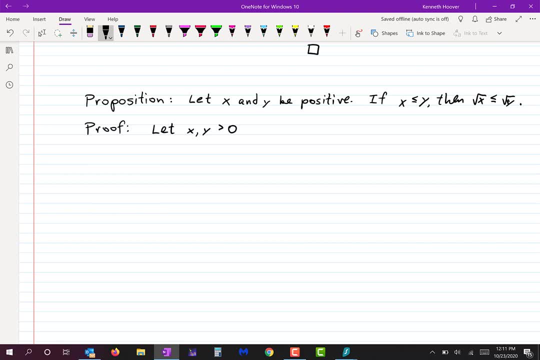 So we can do a couple of options. We can say: let x and y be positive and x is less than or equal to y. Okay, x, and let x be less than or equal to y. Or you can write in two separate lines. 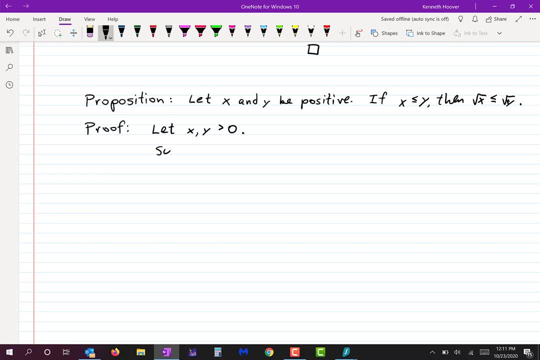 I can say: let x and y be positive Period. Suppose x is less than or equal to y. That's fine, Let's leave it like that, Okay? Now, this is going to be mostly a computational thing, So 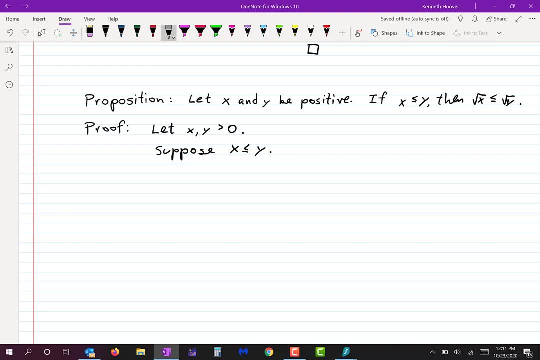 maybe we should work it out as scratch work first. So we're starting with this And we want to get to this. How are we going to do that? Now? I bet there's a lot of people who are saying, oh, just take the square root of both sides. 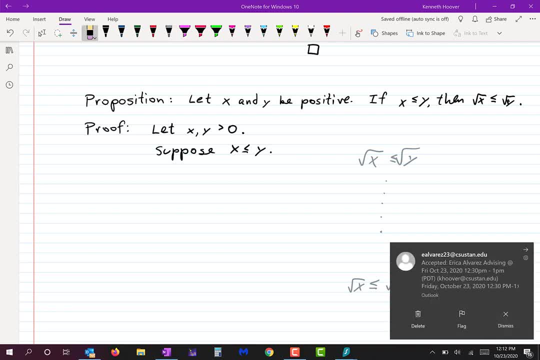 And then we'll be done. Okay, Here's the problem with that. We're trying to prove that that works. We're trying to prove that if you start with an inequality like that and you take the square root of both sides, then the inequality will still be pointing in the right direction. 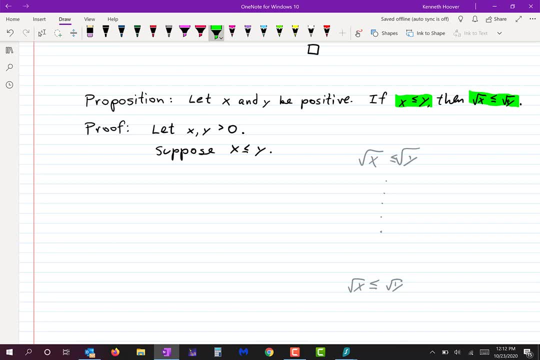 Then the inequality will still be pointing in the same direction. That's what we're trying to prove. So you can't just say we'll start with an inequality and take the square root of both sides. Look, it points in the same direction. 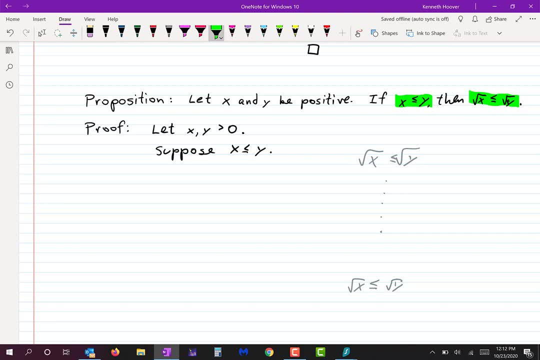 No, because then basically we're just we are doing what it is that we're trying to prove you can do. You see what I'm saying? That would be circular logic. then The whole point is: we're trying to show that if you did take the square root of both sides, 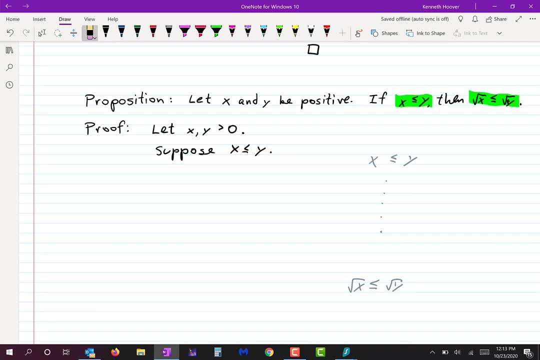 if you did take the square root of both sides, you would still have: the left-hand side is less than or equal to the right-hand side. Okay, All right. How are we going to do that? Well, let's start by doing this. 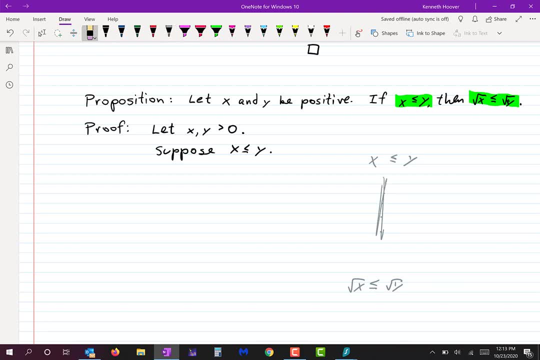 How about if we whoops? how about if we subtract y from subtract y from both sides? This is just scratch work, okay. That's why I'm just writing it off on the side. That would give us that right. 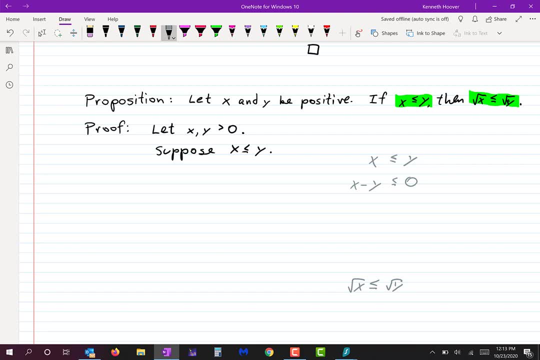 And isn't x the same thing as the square root of x squared? Because of the fact that we are given that x is positive, and so, therefore, I can take the square root of x, and if I square the square root of x, I'll get x right. 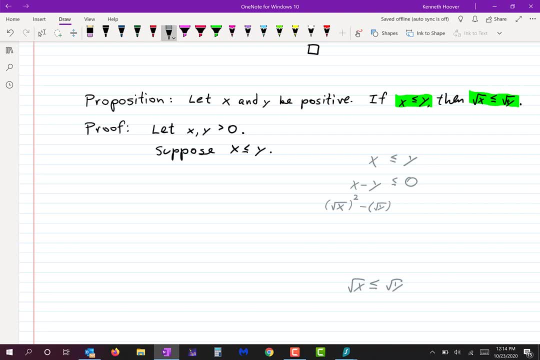 And I can do the same thing with y, correct? And then, since I have a difference of two squares, can't I factor that into this, times this? And then can't I divide both sides By the square root of x plus the square root of y? 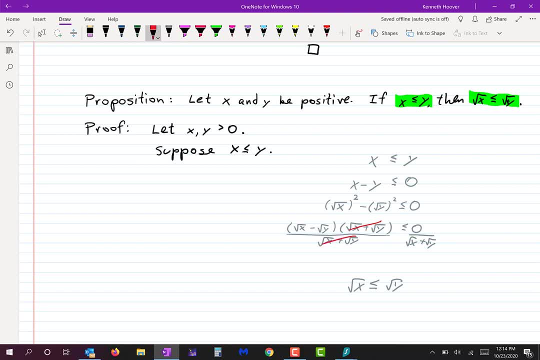 And those will cancel there And I will be left with the square root of x minus the square root of y is less than or equal to zero, Because zero divided by the square root of x plus the square root of y is zero. And I divide it by what kind of number? 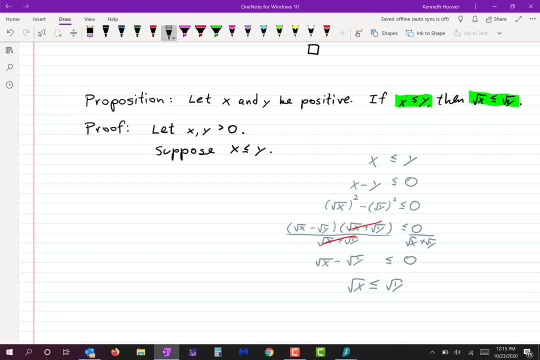 The square root of x and the square root of y are both positive. So the square root of x plus the square root of y is positive. So when I divide both sides by that, the inequality does not change directions. And how do I know I can divide by that? 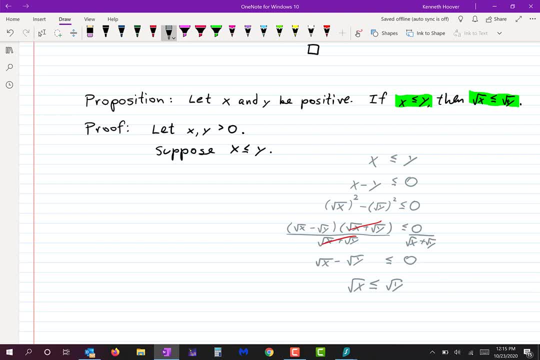 Remember, you can't divide by zero. So if you're just going to come along and divide both sides by something, you have to make sure that that thing's not zero. How do I know? the square root of x plus the square root of y is not zero. 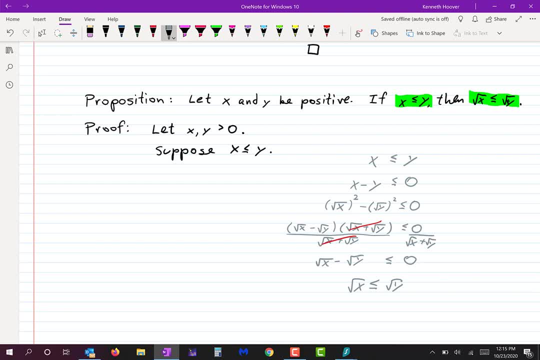 Again, because x is positive and y is positive, So x and y are both greater than zero, So their square roots are greater than zero. So the square root of x plus the square root of y is greater than zero. Okay, Now here's what you cannot. 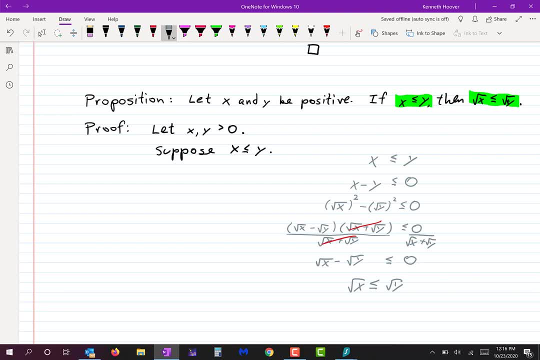 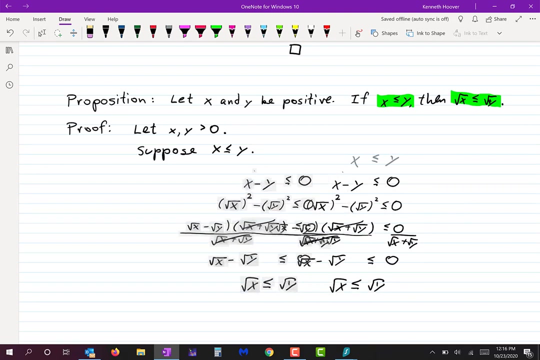 absolutely do not do this And that is to just take that, make it black and put it right there. Do not do that, Not just because it's written a little bit sloppily, but even if I wrote it, even if I wrote it neatly- 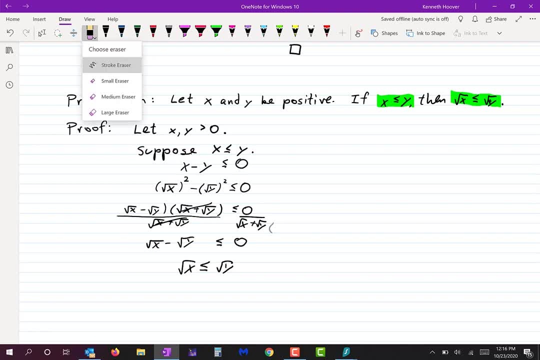 Here, let me show you. So here I'm going to, I'm going to illustrate for you something that I have seen students many times in upper division classes, Well beyond set theory and logic, Doing stuff like this, And it is, in my opinion, 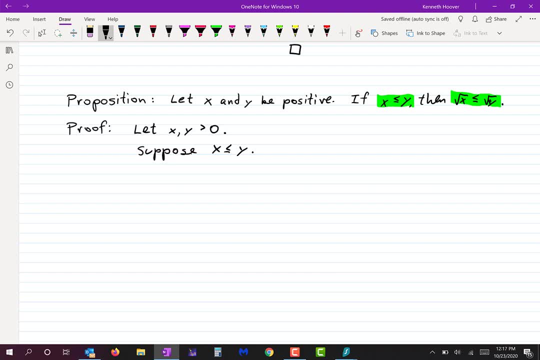 it's not good enough. Okay, A lot of times you'll see stuff like this: Let x and y be greater than zero. Suppose x is less than or equal to y, Then x minus y is less than or equal to zero. 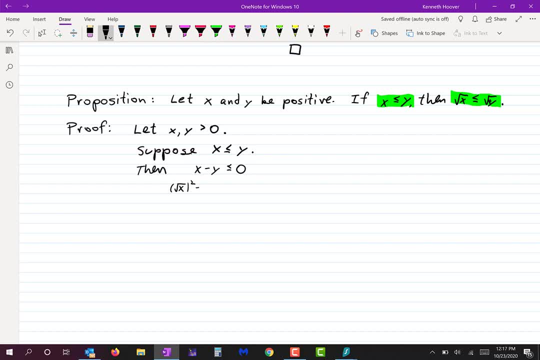 Which means the square root of x squared minus the square root of y squared is less than or equal to zero, Which means root x minus root y times: root x plus root y is less than or equal to zero. And then we divide both sides by: 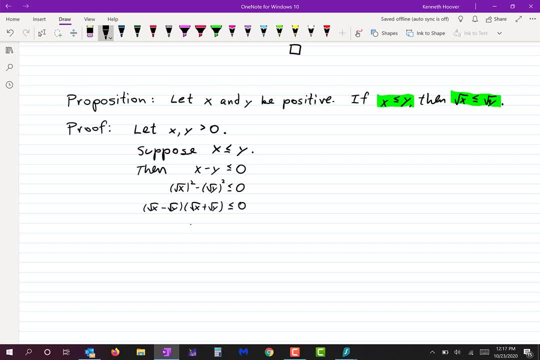 that second parenthesis There, And maybe the person would show that, Or maybe they wouldn't. Okay, Now here's the problem I have with that. Oh, and then sorry. So then what would they do next? Maybe they would say: 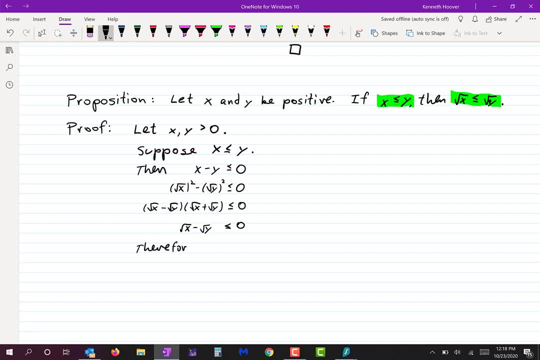 something like: therefore, the square root of x is less than or equal to the square root of y. Because what They add the square root of y to both sides And say, there we go, I'm done, Okay, Now what's the problem with that? 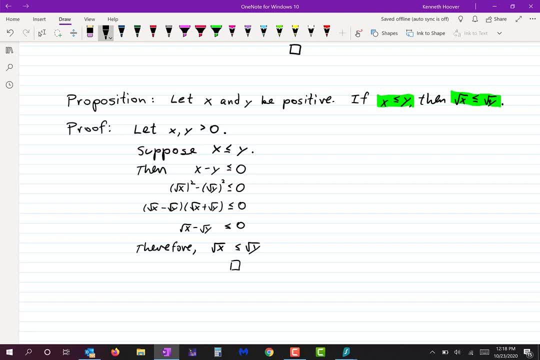 Well, if this was Calculus 1,, that might be okay. Or if this was College Algebra, that might be okay, All right, But we are beyond that, And so we should be writing things more in a more sophisticated way, And what I mean here. 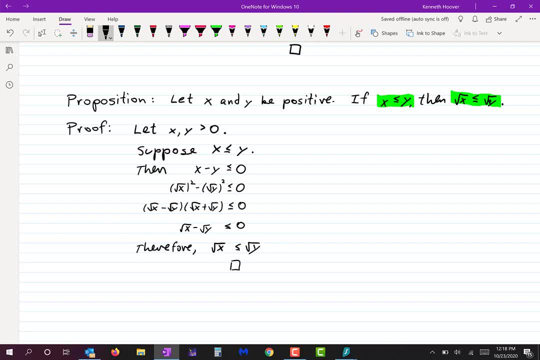 when I say that this isn't sophisticated enough, I'm not talking about the mathematics. I'm talking about putting the ideas together in a coherent string of sentences. Okay, what's the problem here If I asked this student how many lines are in this proof? 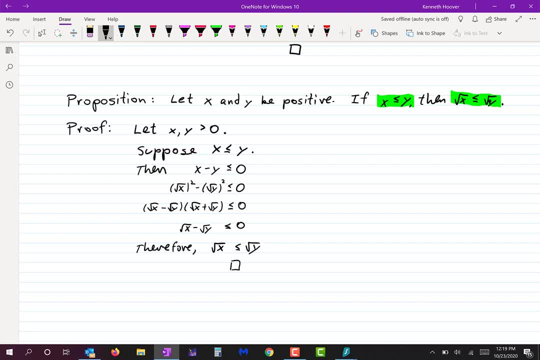 I'm not sure if they would say that there's seven or there's four, But let's just take both of those possibilities. What if a student turned this in and I asked them: how many lines did your proof take? And what if they said there's four lines? 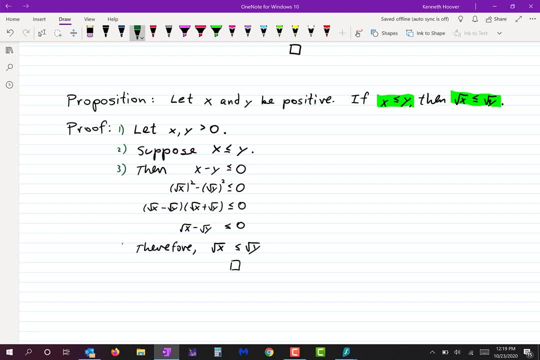 Dr Hoover, can't you see One, two, three and four? Here's what I would say to that person. I would say: absolutely not. This is not one line. If it was one line, then that person is saying this: 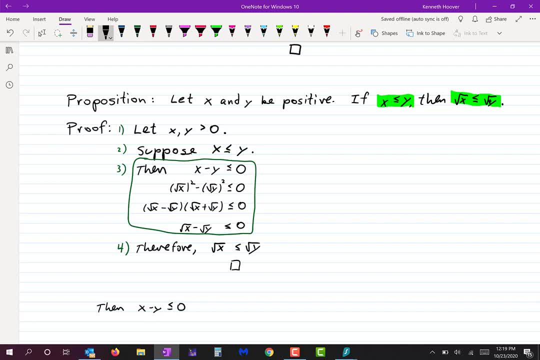 The problem here is that when you ask a student what the proof is and another student must know the proof of the contradiction, then they can observe the proof and be interested in it at all times. All right, well, let's make things clear. 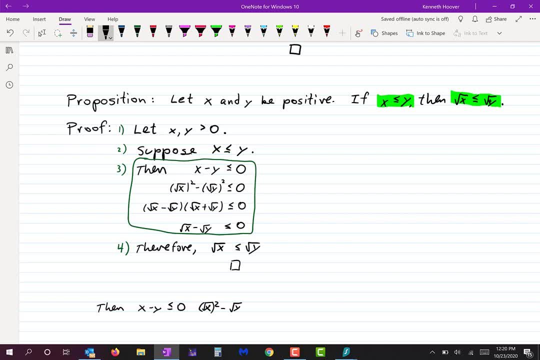 Let's say that I have three lines. I'm going to just say I'm going to use the graph. The graph is the length of the word, because it's the length of the word. It's going to be 5 nesseces. 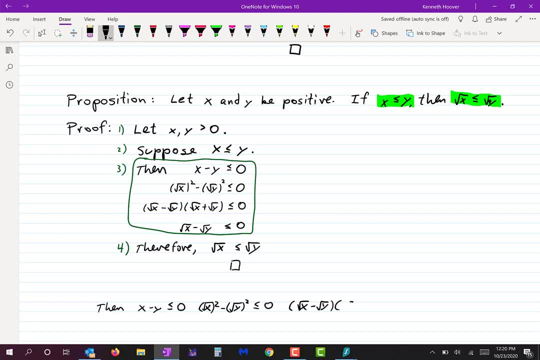 I'm going to say that the third line is the length of the word. Let's say, the second line is what this girl said. I'm going to put the next line and the third line is what this girl said. So that's what I'm going to do. 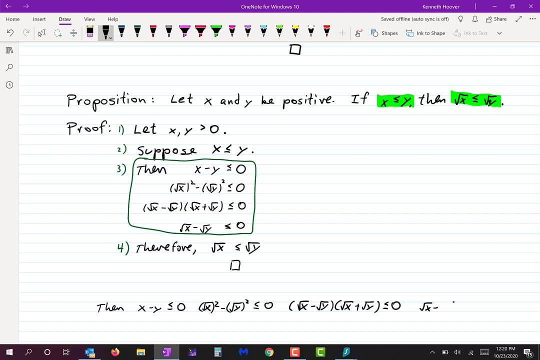 And I'm going to just go along with this. Look at the graph. that's what the person is saying. if they're saying that that green box is one line, then here's what it is. only they. they've written it going down instead of going across to save room on how long it is. now look at that. read it. 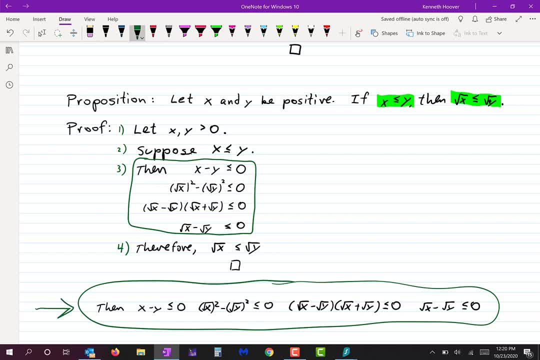 out loud. does that make any sense to you? it shouldn't, because why? it's for separate inequalities with absolutely no wording or anything separating them. listen, I'm going to read it out loud. then: X minus Y is less than or equal to 0. the square root of x squared minus the square root of y squared is less than or: 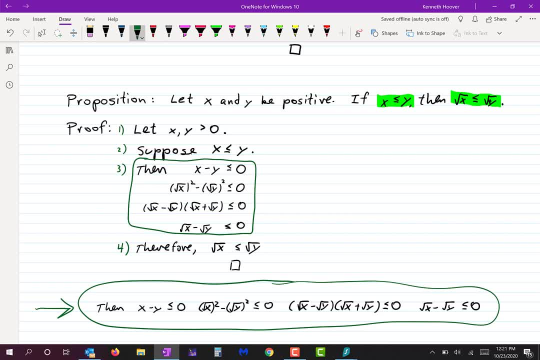 equal to 0. the quantity square root of X minus root Y, times root X minus root Y is less than or equal to 0. root X minus root Y is less than or equal to 0. is that a coherent sentence? no, it's not so. I mean. it can be made into a coherent sentence by putting things like commas. 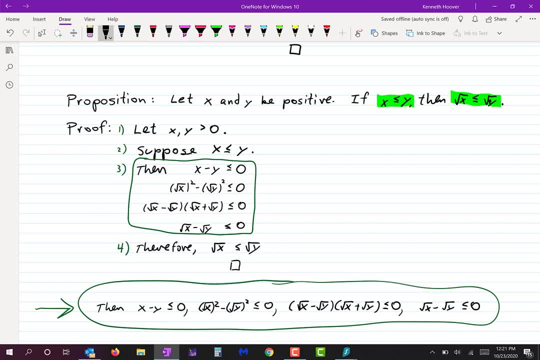 in between and some sort of wording to transition from one idea to the next, like so or something like that. but I still have the problem that sounds like a run-on sentence because you've got four different ideas all there in the same sentence. so the truth of the matter is, the point I'm trying to make is that 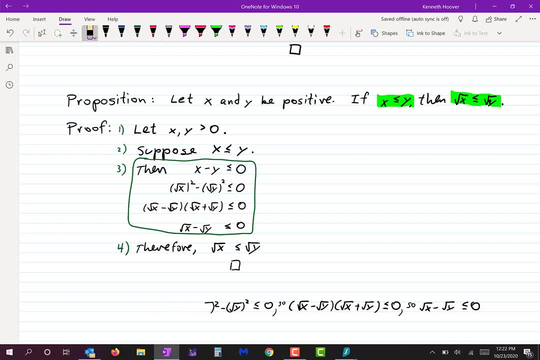 that in the green box up there is not one line, it's actually four different lines, and the truth is that that proof is a seven line proof. ok, so let's number them properly. not because you need to number your lines, you don't on numbering them because I'm trying to make a point here. 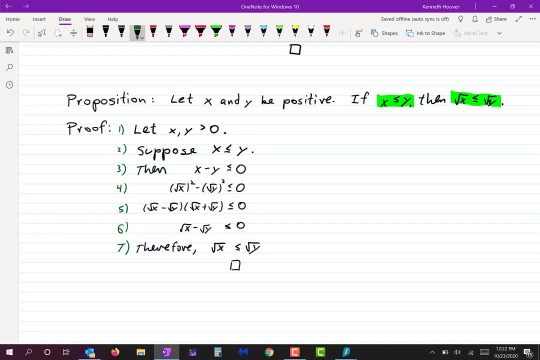 ok. so now, now that I got the student to understand that this is four different lines here, now I say to the student: can you see the problem I have with lines four, five and six? ok, and this is where the word sophisticated comes up. we are well beyond calculus one, we are well beyond college algebra. we 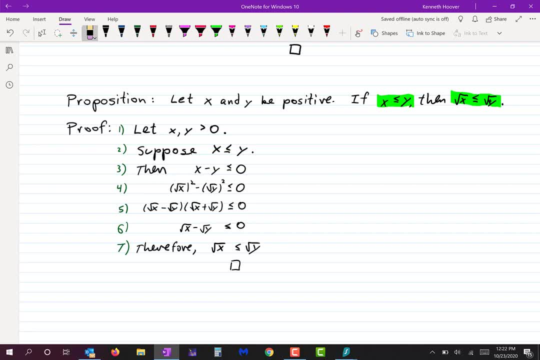 are math majors and we are writing proofs, so we should be a bit more sophisticated than a college algebra student. our proofs should consist of complete sentences, and I'm not just being picky there. ok, that's the truth. our proofs should consist of complete sentences. so what's? 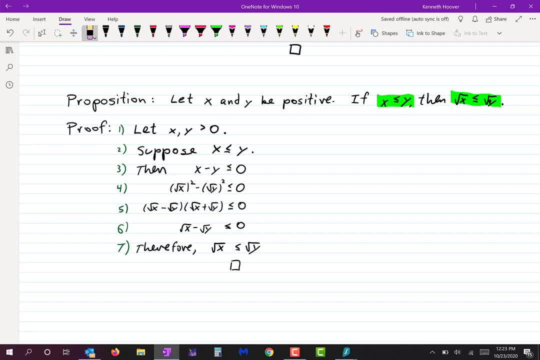 wrong with line four, five and six? well, what I have wrong with them is where's the word that starts each sentence? you see, there's a logical relationship between those lines, isn't there, along with line three, isn't it that this causes this to be true? right, like, like I could ask the student, I can ask. 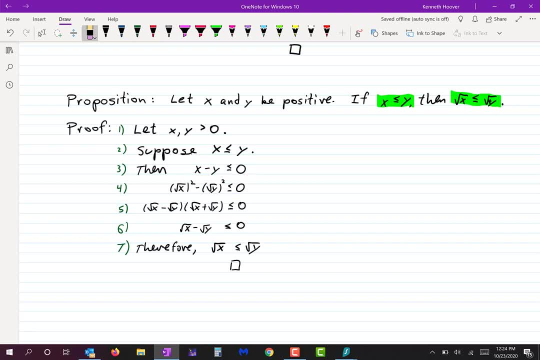 the student: well, where did you get line four from? how do you know? the square root of x squared minus the square root of y squared is less than zero. and surely they would say: well, because of this right here. so there is a cause and effect relationship that causes that right. so then shouldn't there be some sort of logical words? 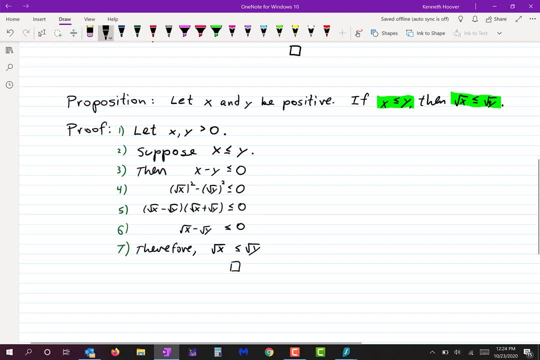 showing the cause and effect relationship. in other words, what I'm trying to get to is: how about the word then? because this is true, then this is true, ok, and that's the same problem I have with lines five and six. Now, as I have said, it sometimes sounds awkward to say then, then, then, then, then. so certainly. 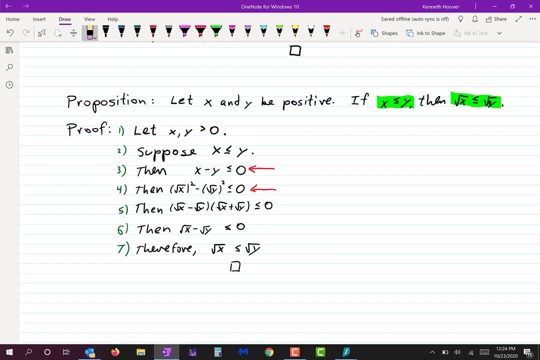 you can do what I have been doing with you guys in these examples and use a mixture of different words like then, hence thus, things like that You can. even this one sounds unsophisticated to me, but every once in a while, if I get, 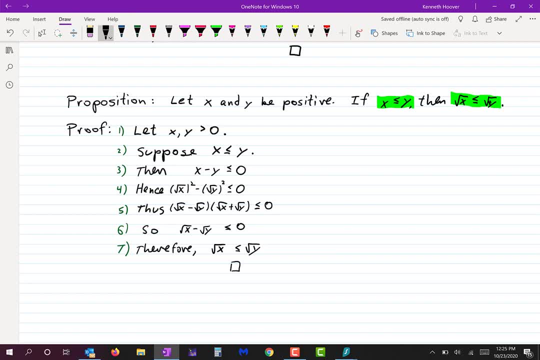 tired of saying then, hence and thus, you can even say so. Or if you wanted to get even fancier, you could say: as a consequence, Consequence, Consequence. I think that's being taking too much room. I wouldn't want to write out as a consequence, but you certainly could if you wanted to. 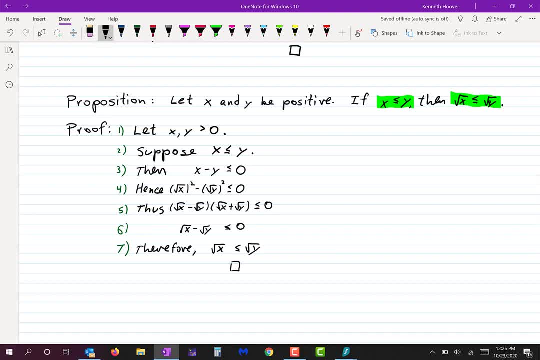 My rule of thumb is: once I've burned through, then hence and thus then I feel like, okay, now it's been long enough, I can go back to then again without feeling like I'm being repetitive. You see what I'm saying. 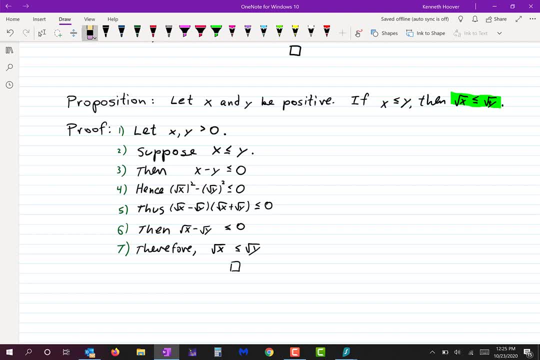 I'm trying to give you guys a glimpse into my way of thinking when I'm writing a proof. Now, that's much better. One other thing, though. I think it is entirely reasonable to somebody to see how we're getting from here to here. 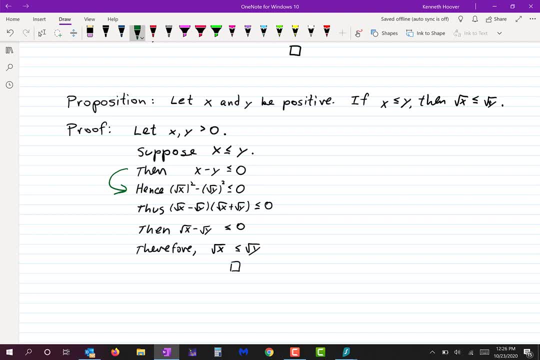 I don't think it should need to be explained. Okay, I think it is entirely reasonable to assume That somebody can get from here to here without any extra explanation. I just factored is all I did Now. from here to here, I'm on the fence. 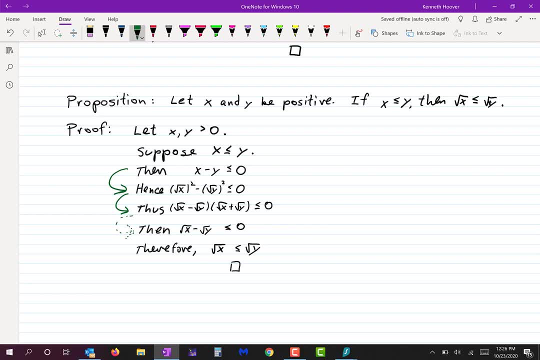 I feel like, yeah, that's reasonable. I mean, what did I do? I divided both sides by the square root of x plus the square root of y. I think it's reasonable to think that someone would be able to follow that. 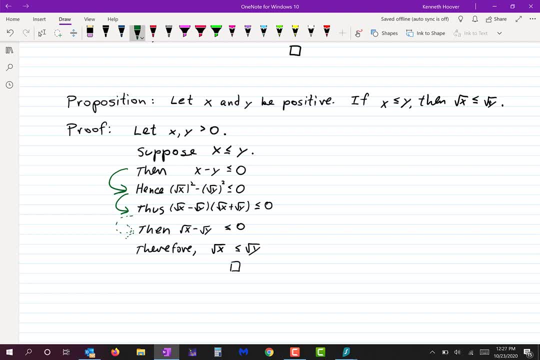 However, at the same time, I don't think it is unreasonable to say: maybe I should explain what I just did. I don't know. That's sort of a gray area there. You know what I mean. I actually did something, you know, not a tiny step. 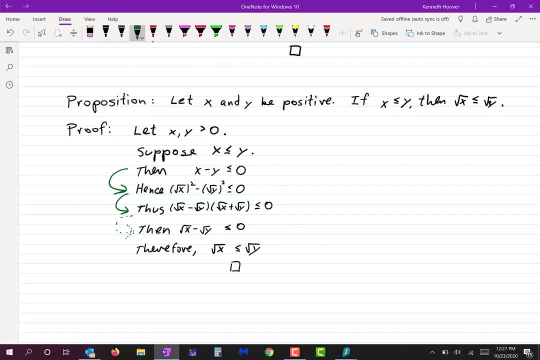 I divided both sides by the square root of x plus the square root of y, But when somebody's reading this, I suppose I'm a little worried maybe they won't see that, because it just looks like the square root of x plus the square root of y just disappeared, right. 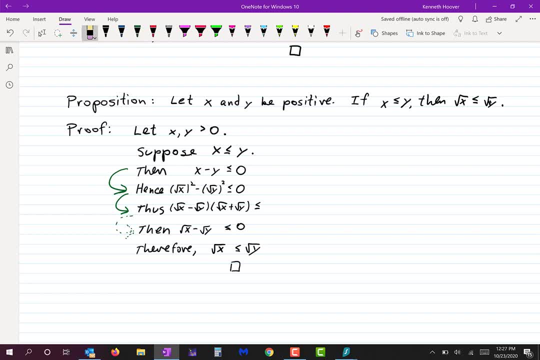 If this was a two, let's say here- this is the point I'm trying to make- Let's pretend for a second that that was a two. Then here we would have two over root x plus root y, And I would say: anybody who's reading this should be able to follow what I just did. 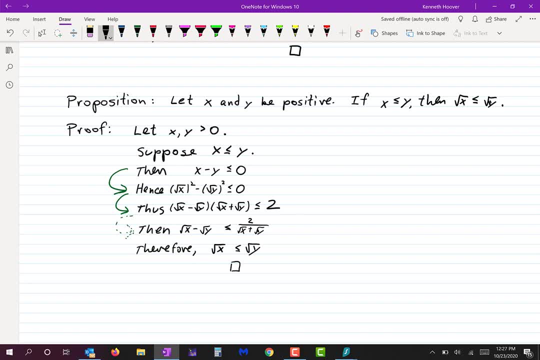 I just divided both sides by root x plus root y. But the fact that that's a zero means that here we had zero over root x plus root y, And since zero divided by root x plus root y is zero, then we just have this. 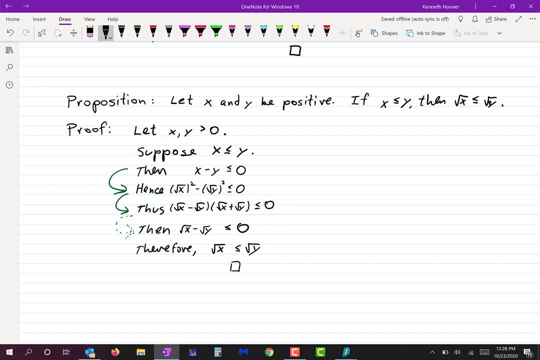 And somebody possibly might get confused because they might think where did the root x plus root y go to? Okay, So I feel like maybe there's some explanation that it might be a good idea to throw in there, Like maybe this: Maybe go ahead and write zero over root x plus root y. 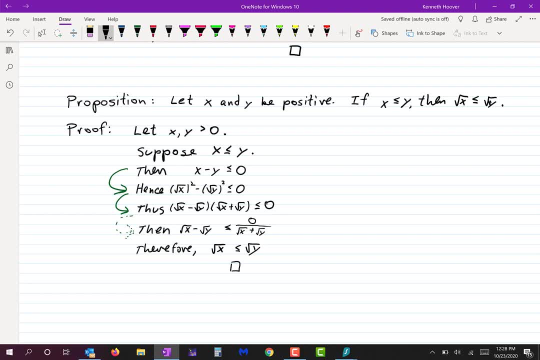 so that everybody can see exactly what mathematical step I just did And then say which equals zero. I think that would be better. Okay, And there's something else too. There's another thing that's very important there that can't get overlooked. 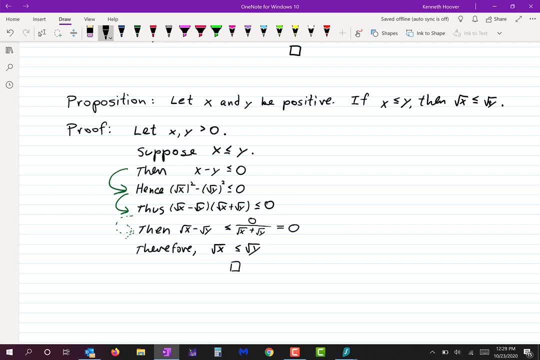 and that's the inequality. What sometimes happens when you divide an inequality on both sides: Sometimes it changes direction. Did it change direction here? No, I think you should point out why it's not changing direction, because I think that is a very reasonable question. 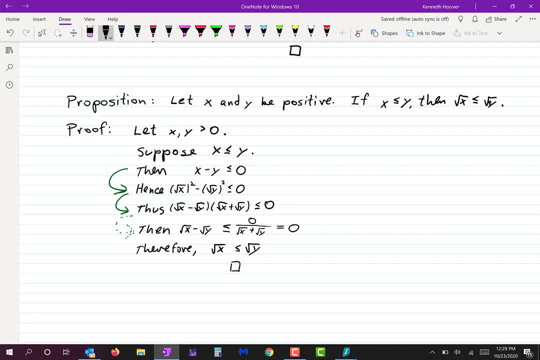 How do we know that? it didn't change direction? So we should point out, since square root of x plus square root of y is positive- And again this is up to you totally, but personally I could see myself putting that before the calculation- 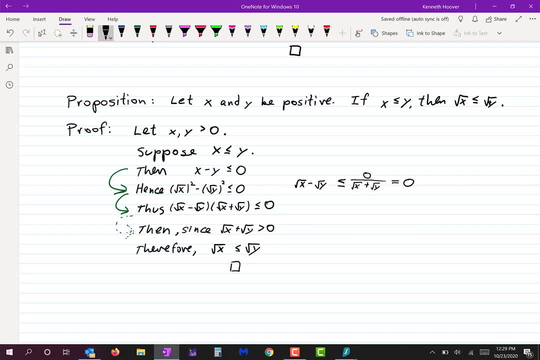 But that's entirely just personal preference. Okay, Do you think I need to explain why the square root of x plus the square root of y is positive? I don't think so. I would expect someone to know that if I have pointed out that x is positive. 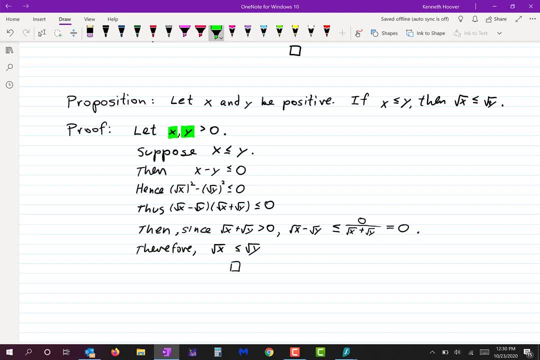 I would expect someone to know that x is positive. I would expect someone to know that x is positive. I would expect someone to know that x is positive, And if x and y are both positive, I would expect them to be able to know then that their square roots are positive. 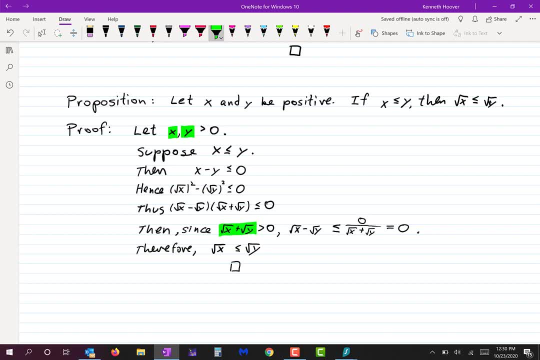 and I would certainly expect them to understand that when I add two positive numbers together, I get a positive number. So I don't think I need to explain why root x plus root y is positive. But I do think that when you divide both sides of an inequality by a number, 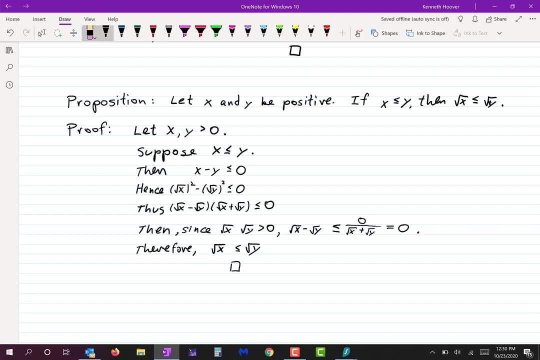 and the inequality does not change directions. I think I should point out why it did not change directions. Now, if it was just the number 5 that I was dividing by, then I wouldn't say: because 5 is positive. That's too trivial. 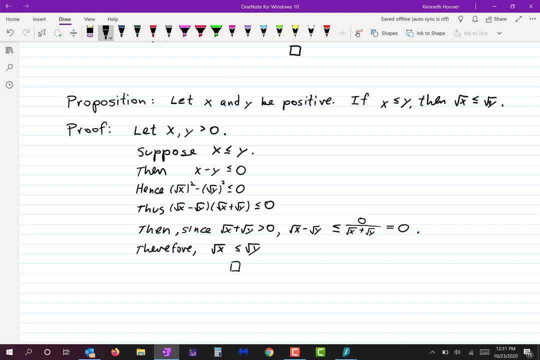 But root x plus root y, I think I should say, because that's positive. then when I divide both sides by that, the inequality doesn't change. Okay. And then what's my reasoning for this line, and should I point it out? 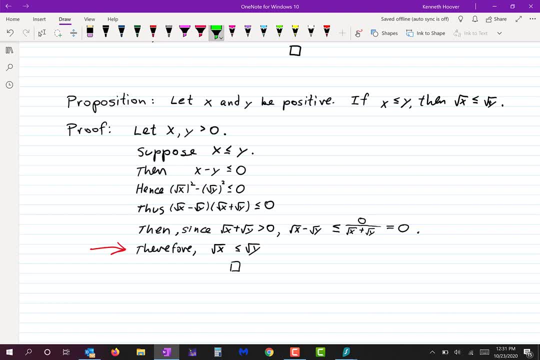 I don't think we need to point, I don't think we need to point out our reasoning, but here it is. It's because I just took this, which is less than or equal to 0, and I just added root y to both sides. 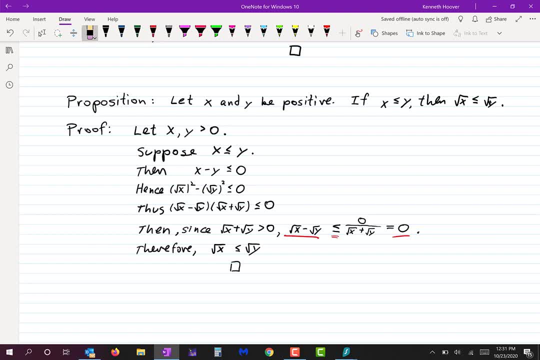 Okay, Remember my rule of thumb. If all you're doing is algebra, I don't think you need to point out, I don't think I need to say by the addition property of equality. That's technically the rule that says you can. 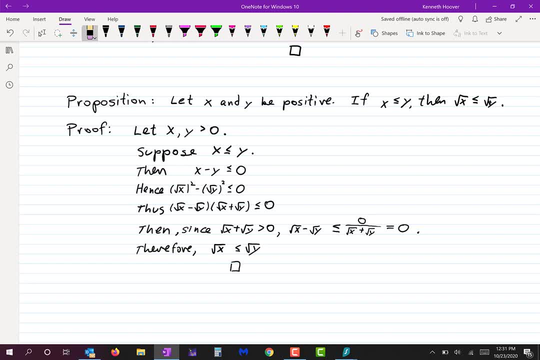 add something to both sides. Okay, All right, So that's really a pretty short proof, but I think that was a really good one, because I was able to illustrate for you mistakes that people often make by essentially doing what scratch work. Remember what I had written in gray. 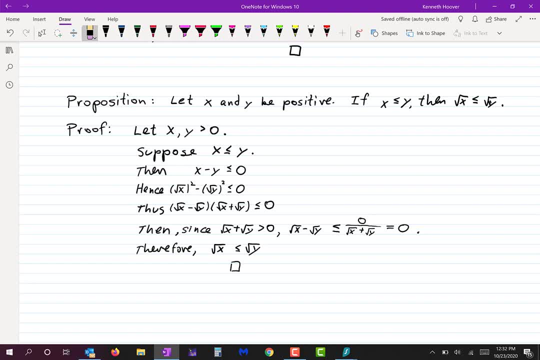 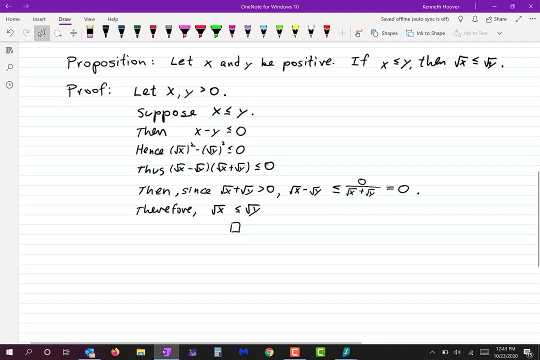 That was scratch work, And a lot of times people will take that scratch work and then just put it in the proof and say the scratch work is my proof, without even realizing that that's what they're really doing. Okay, one more, And then we're going to start moving forward. 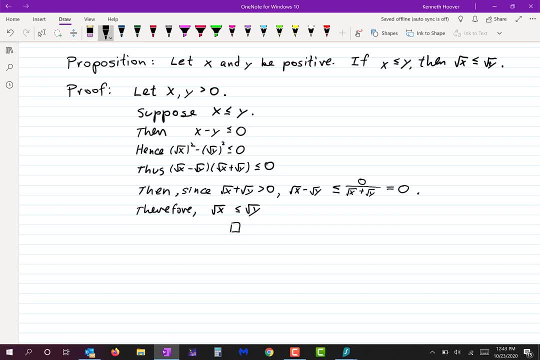 after that to the next section. Let me fix my microphone, Okay. So proposition: This one will also be a short one. This one will be similar to the one before. Okay, We're going to prove that if x and y are positive real numbers, 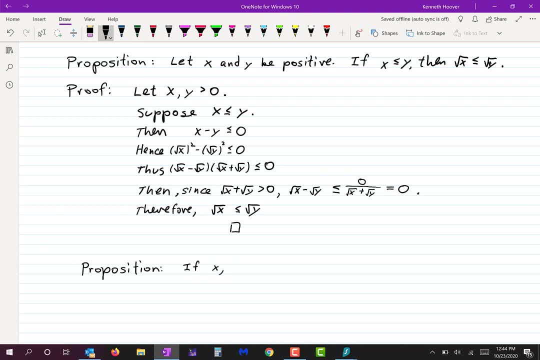 Okay. So if x and y are positive, Whoops. Okay, You don't have to say real numbers, but you can. But when you say one number is bigger than another, then we know it's not complex or imaginary, because there's no such thing as bigger than. 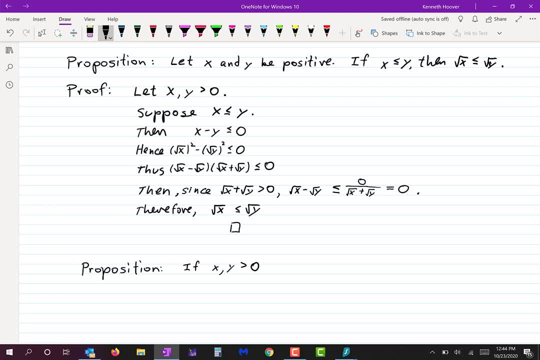 There's no such thing as a number between complex numbers. Okay, And so therefore it's implied that they're real. Now, if I wanted them to be something more specific, like rational, then I would need to say that, Okay, But if they're just real, 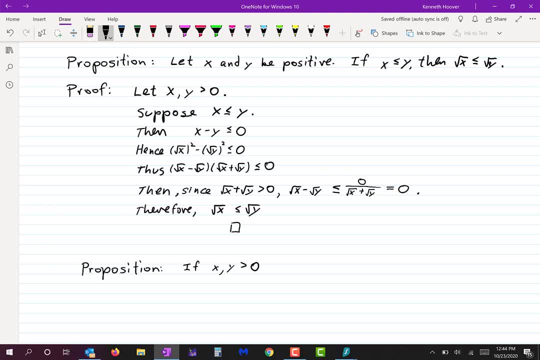 that's the largest category that we're going to be worrying about. Okay, So you don't have to point that out By saying x and y are greater than zero. I'm saying they're positive and it is implied that they are real. 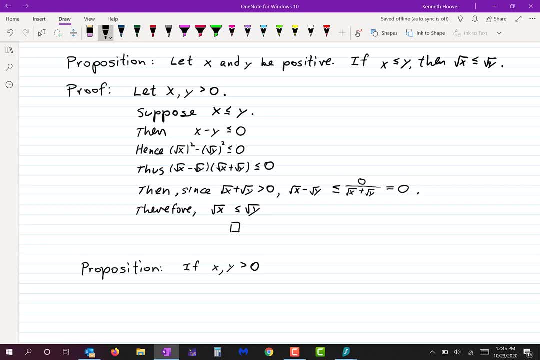 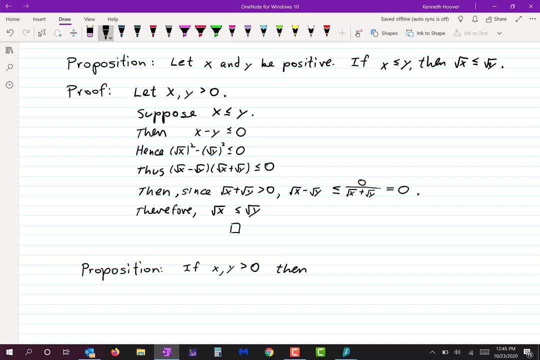 Okay, All right, So anyways getting on. If x and y are positive numbers, then two times the square root of x times y is less than or equal to x plus y. All right, Let's prove that. And this would be a similar type as the one up above. 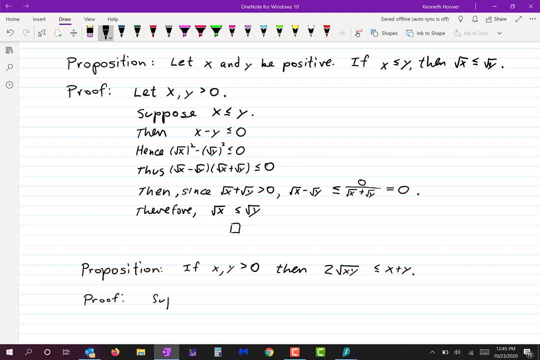 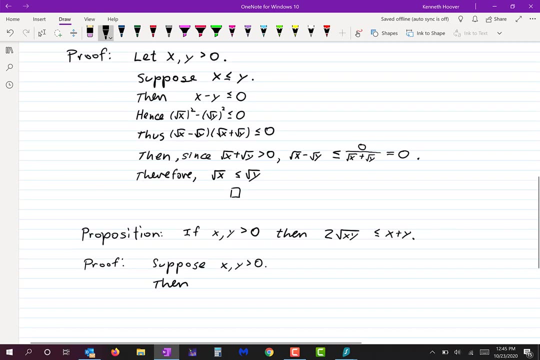 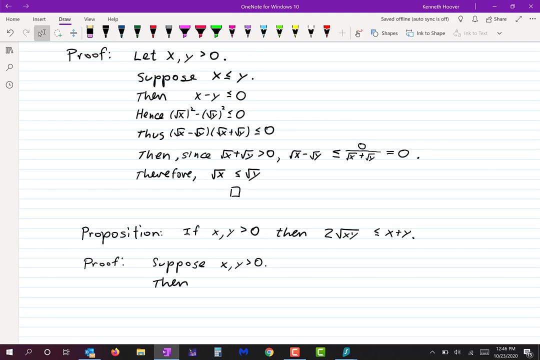 Okay, So suppose x and y are positive, Then what can I say about that? Okay, So here's what I would say next. Now, this is assuming I've already formulated a plan. I mean, that's what you have to do first. 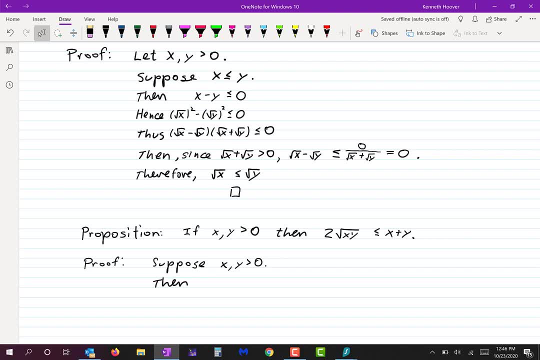 When you're proving something you don't oftentimes figure out as you're writing it down. How would you do that? When a composer writes a song, do you think that they are figuring it out as they're going? Probably not. They have to keep stopping. 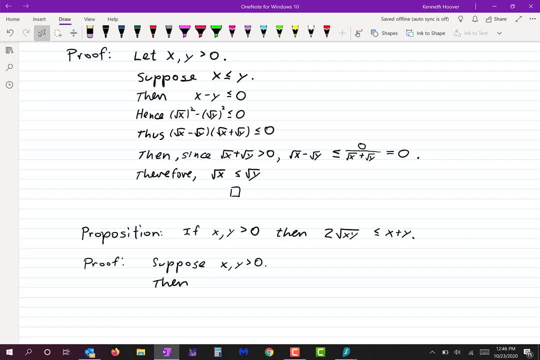 and thinking about what they want next, Right? So probably you need to figure this out with some scratch work beforehand, And some of them are simple and some of them are really, really hard. Okay, But you do not. you don't usually figure out a proof. 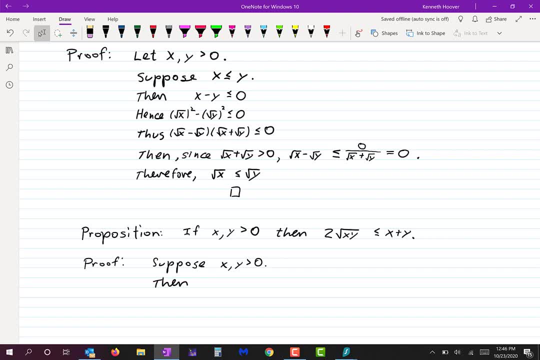 as you're going, as you're writing the proof, unless you've just had an awful lot of experience with it. Okay, So here's what I would do. Let's say we want to get to this right. Let's do some scratch work. 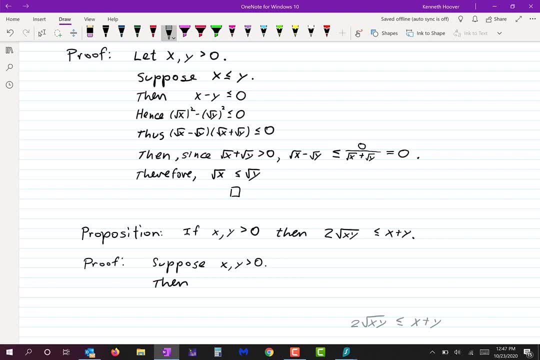 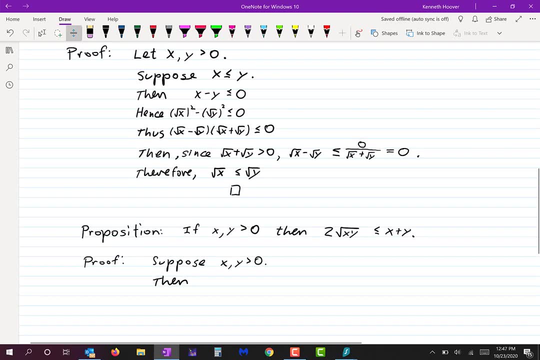 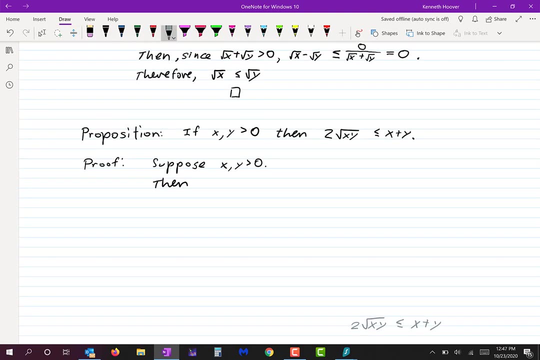 We're trying to get to that. I'm not sure yet if this will yield anything useful, but it's just an idea. How about if we subtract 2 root x, y from both sides? I'm just working my way up, Okay. 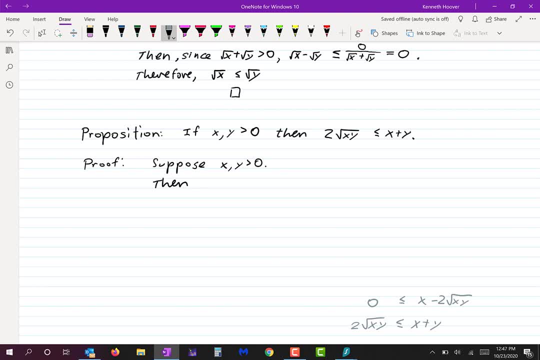 And let me put it in the middle: Okay, Do you see how that might be helpful? Because that's actually the left-hand side, is factorable. See, isn't the left-hand side? look, I'm sorry, not the left-hand side. 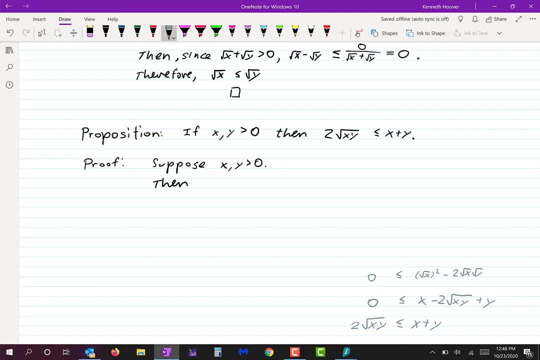 I meant the right-hand side. Okay, Isn't this? it's the same thing as that, And so, therefore, isn't it equal to square root of x minus square root of y squared. And don't forget, don't we know this is true. 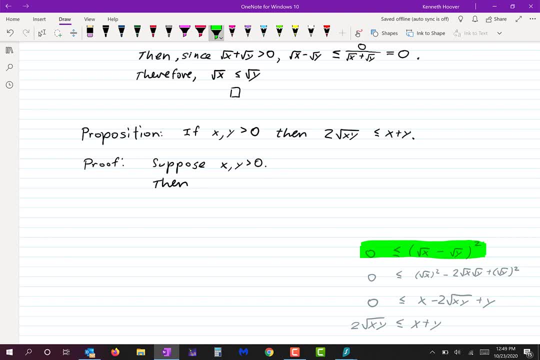 Because any number squared is equal to or greater than 0.. It doesn't even matter what's in those parentheses, does it? Any number squared is equal to or greater than 0.. And this whoops. and this equals this, which equals this. 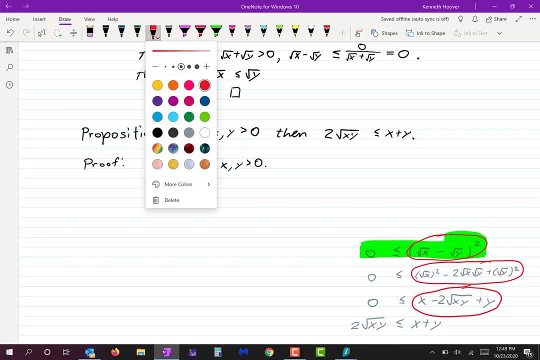 which equals this. So this being true, so this being true means this is true, which means this is true, And then if we subtract, I mean add to root, x, y, to both sides, and then we'll get this and we'll be done. 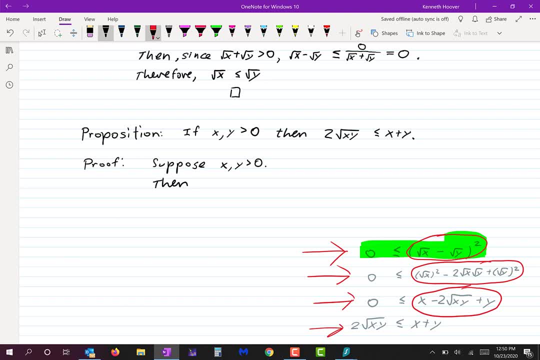 Right. So that's certainly one way to do it. I could say: suppose x and y are positive, then the square root of x minus the square root of y, quantity squared is equal to or greater than 0.. And then how about if we? 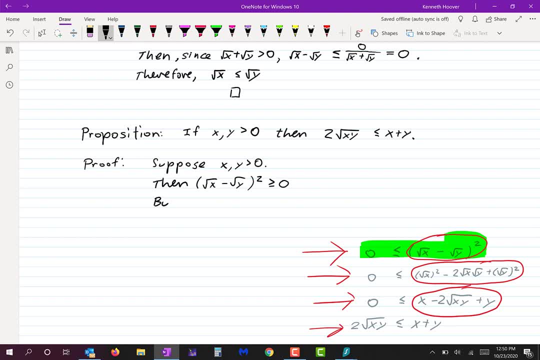 how about if we do this and say: but the square root of x minus the square root of y squared minus the square root of y squared equals x minus 2 root, x, y plus y. So x minus 2 root, x, y plus y. 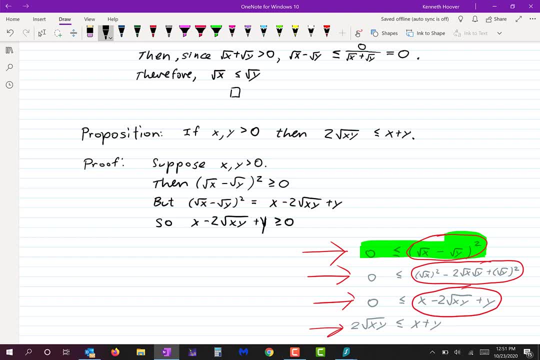 is equal to or greater than 0.. You see how I'm explaining that. Hence, x plus y is equal to or greater than 2 root xy. And all of that was just basic algebra. That one was actually really easy, wasn't it? But do you see how every single line is a complete sentence? 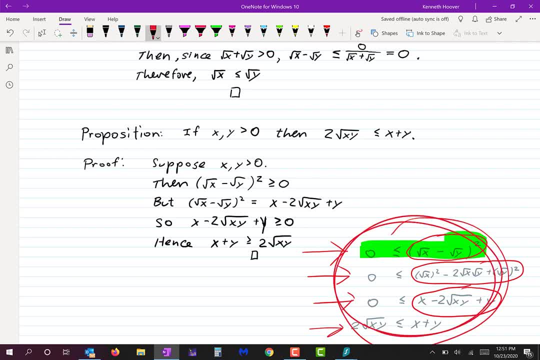 I didn't just write this out here like that and say: here's my proof, did I? It's readable. Now I would like to show you one other way of doing this. If you're reading in the book, which you should be, reading, the book. 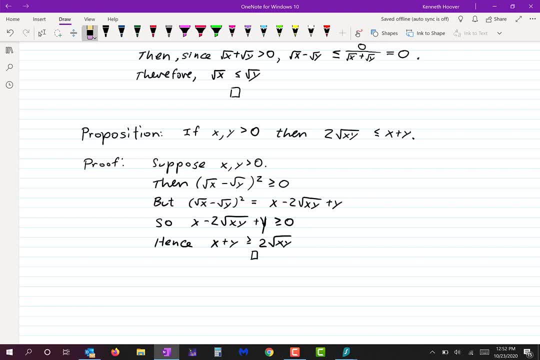 you'll see that I've done it slightly different than they did. What they did in the book was, instead of starting here with the square root of x minus the square root of y squared, what they did was they started with just x minus y squared, And of course that's. 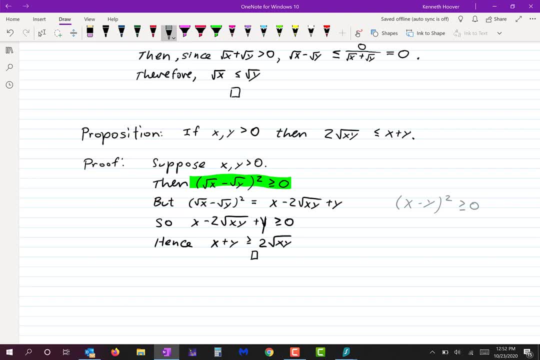 greater than or equal to zero, because it's something squared. And then they worked that out to get x squared minus 2xy plus y squared, And then what they did was then they added 4xy to both sides, So the negative 2xy in the middle becomes positive 2xy. 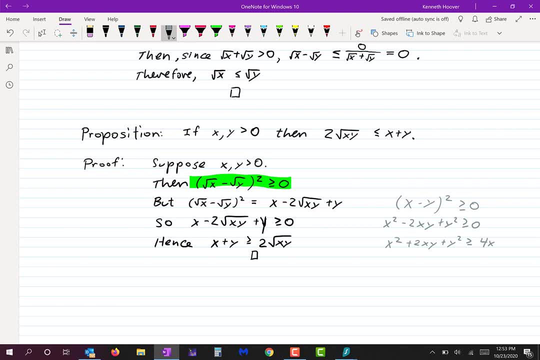 And on the other side, you get 0 plus 4xy, which is 4xy. And what is that? on the left, The left factors into x plus y squared, And then what they did was they took the square root of both sides. 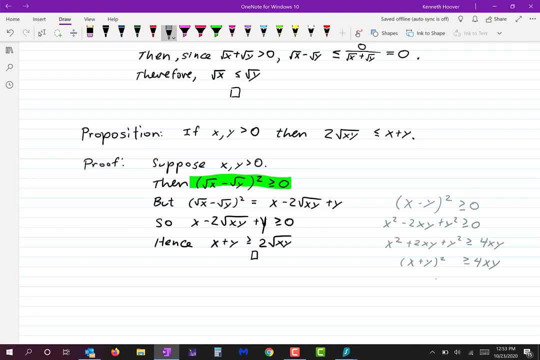 Now a couple things to say about that. So then they took the square root of both sides. A couple things to say about that. What is this? It's x plus y, right y. This is really important Is the square root. 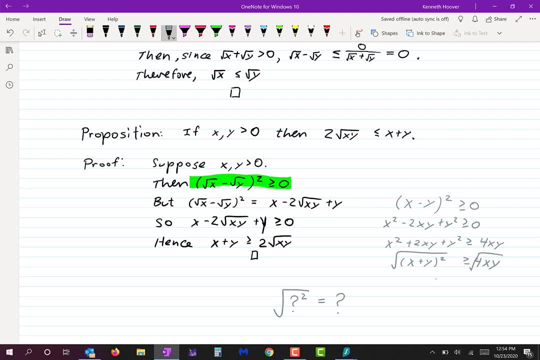 of something squared equal to that thing, that's being squared inside the square root. The answer is no, it's not. It is equal to the absolute value of that thing. So this right over here is technically the absolute value of xy. But since x and y are both positive, 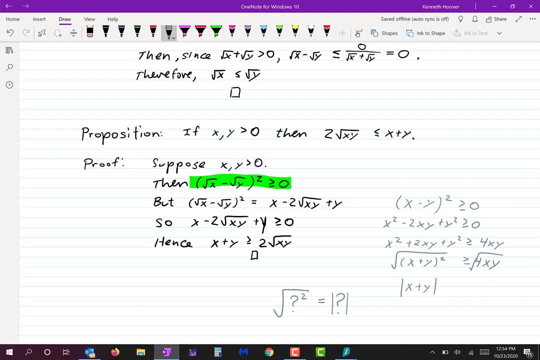 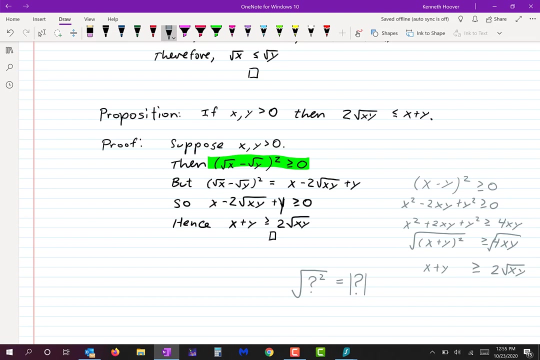 then x plus y is positive, and so the absolute value of xy is xy. Okay, And what do we have on the other side? We have the square root of 4 is 2.. Square root of xy is square root of xy. Now, how do I know? the inequality does not change directions. 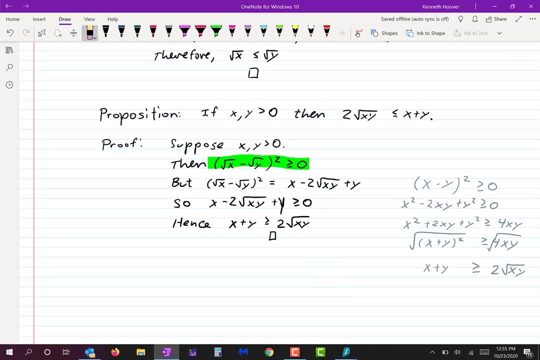 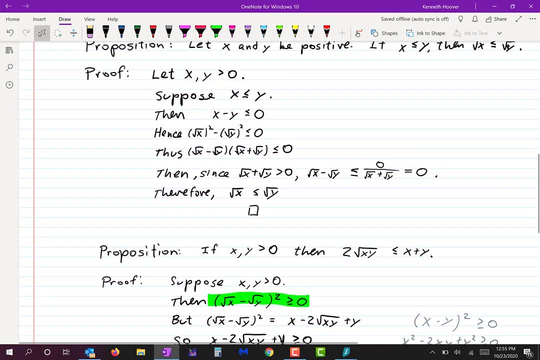 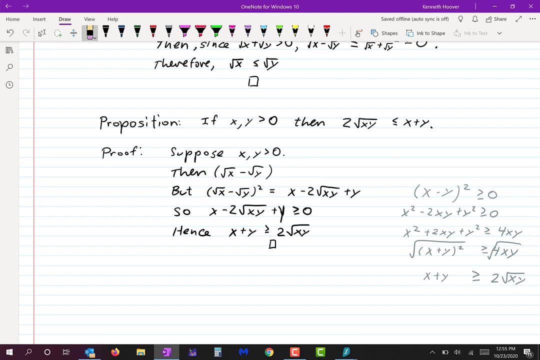 when I did the square root of both sides, Because that's what we proved in the previous proposition. That's why, Okay. so if you were wanting to do the proof that way, let's go ahead and do that. Okay. so I would say: suppose x and y are positive. 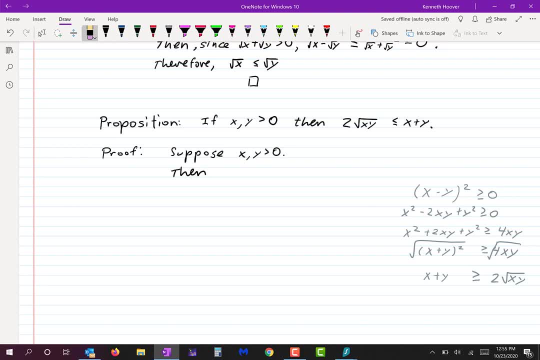 Then, and since this factoring and stuff is a bit easier because there's no square roots in any of this up here, So I think it's even easier to follow. So what I would say is I would actually combine those two things, those two lines, I circled, and I would say then: 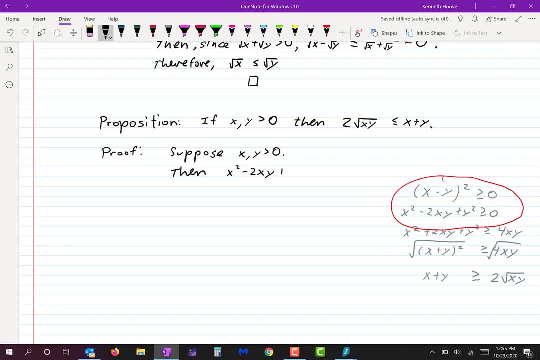 x squared minus 2xy plus y squared, which equals x minus y squared, would be equal to or greater than 0. Because anything squared is zero, So anything squared is equal to or greater than 0.. Okay, And then we add 4xy to both sides. 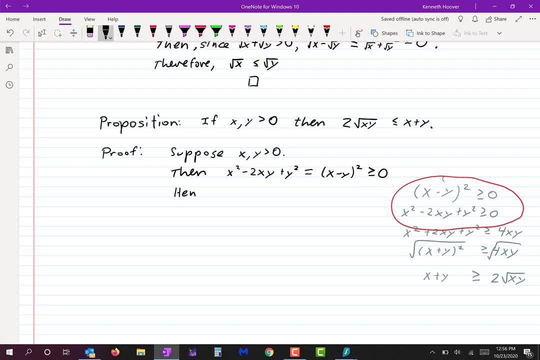 Now we could write this: What did I do? I added 4xy to this, And I got that. And on the right hand side, I added 4xy to 0. And I got that. Now here's the thing. 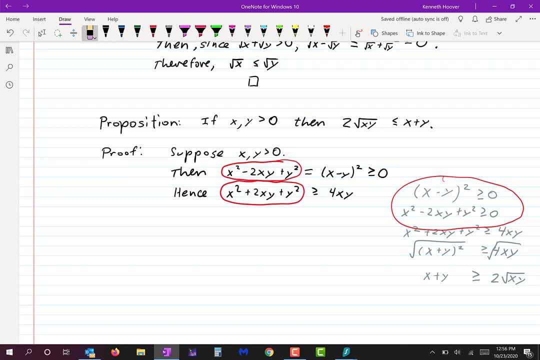 Any reasonable person should be able to follow that. However, look at the left hand side. The difference is simply the minus becoming a plus, And it is so easy for somebody's eyes to look right over that And to totally not see it. 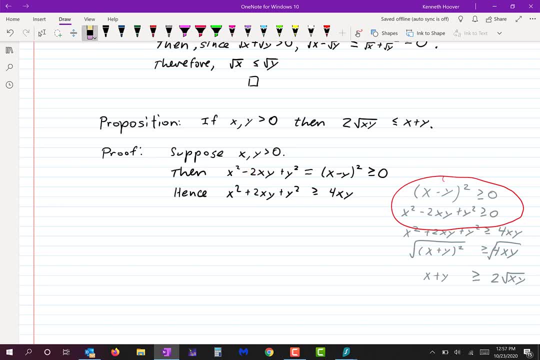 Okay. So even though I think a reasonable person should certainly be able to follow that algebra, I do think, since visually the left hand side is such a minor, minor difference, I think we need to be understanding of the fact that people might not see what it is that we just did. 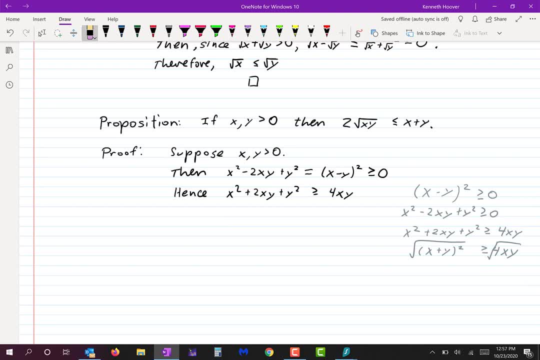 And so it's not a bad idea here to just head off any confusion before the confusion happens And go ahead and say: okay, look, we're going to add 4xy to both sides. So instead of saying hence that, let's actually say: 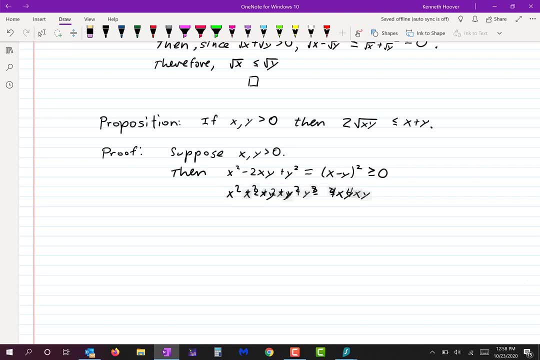 by adding 4xy to both sides comma, we get okay. So we basically just headed off any confusion before it happened. Okay, All right Now. what do I want to do with that? Well, the left hand side there equals what? 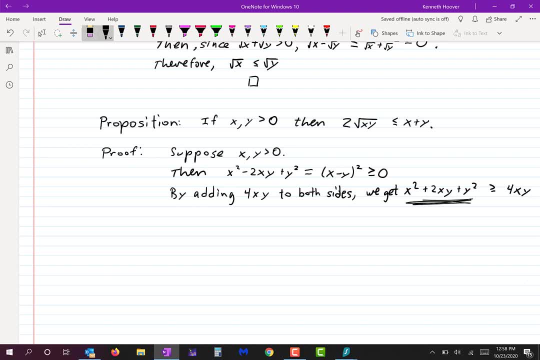 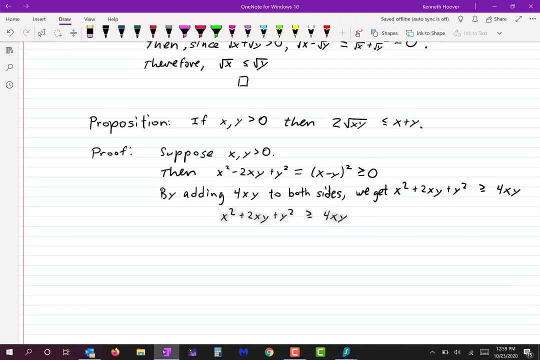 x plus y squared Right. Well, again, like I did in the previous line, I mean, that's such simple algebra. We can go ahead and and actually just do this. I think I don't. I don't think this is at all too much to say at once. 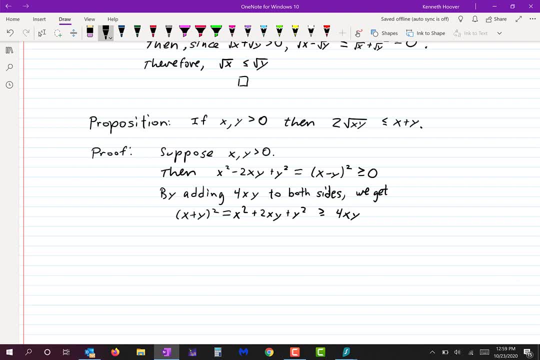 I think we can say that all at once: Okay, Okay, And now what? What should we say to do? We do the square root of both sides right. And how do I know that that will not change the inequality? Because that's what we proved in the previous proposition. 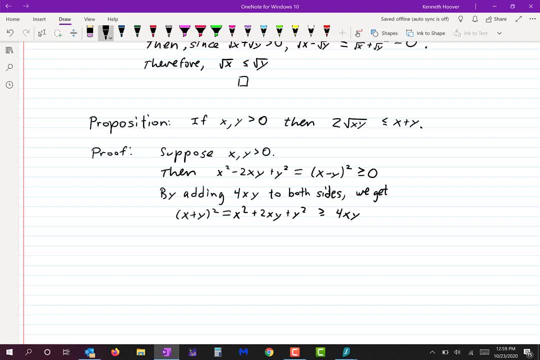 Okay. So I would finish it off like this. I would say thus, or let's say therefore, since I believe this is probably going to be my last line, Therefore, And but there's still a lot to say. Remember, we did, I did, the square root of x plus y, squared right. 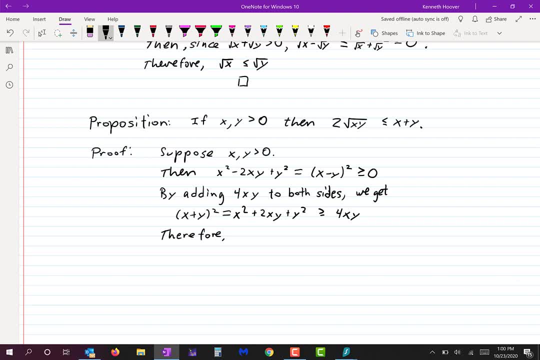 And I got x plus y right. So let's let's show that x plus y equals the square root of x plus y squared, Which is equal to or greater than the square root of 4xy. Which equals what? Which equals 2 root xy. 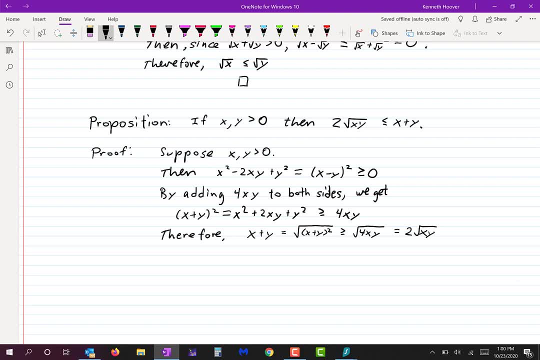 Now, where's the important part of that? I mean, it's all important, but where's the where's the real key? The real key is this right here, correct? How do I know that's true, Because I took this less than or equal to that. 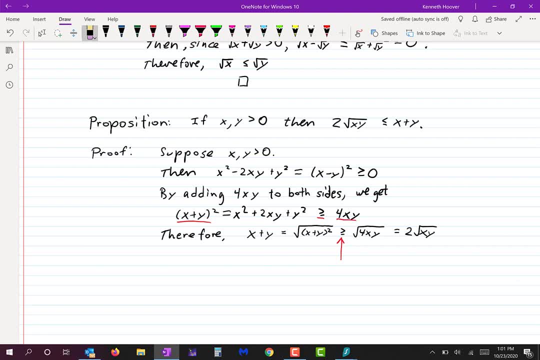 And we did the square root of both sides. And how do I know that that works? Because that's what we proved in the previous proposition. So I will say: by the previous proposition- If it's not the previous one but was one you know, back a few propositions- then what should I do? 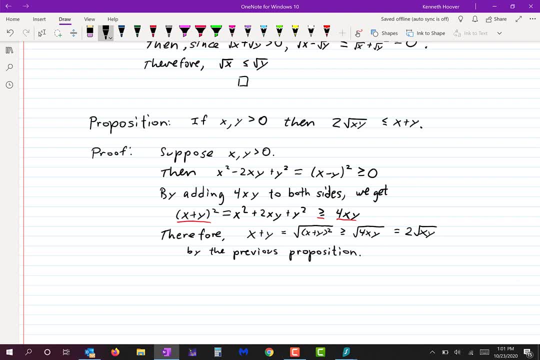 Then I should number my propositions Here. I could say by proposition number such and such, Okay. Or if it was an important theorem that had a name, you could say by this theorem with this name, Okay. I would be really impressed if somebody even pointed out what I said earlier. 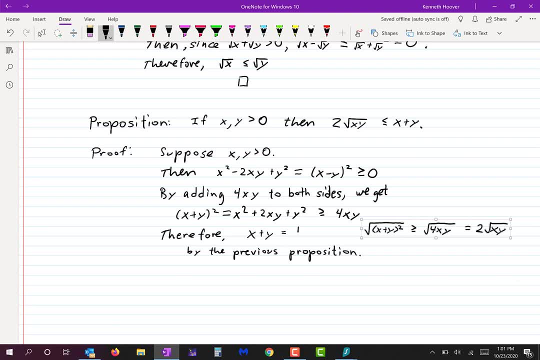 About the absolute value of x plus y. If I saw that I would be impressed. I'd say, wow, that person really knows that the square root of something squared equals the absolute value. Okay, Alright, we did many, many examples. 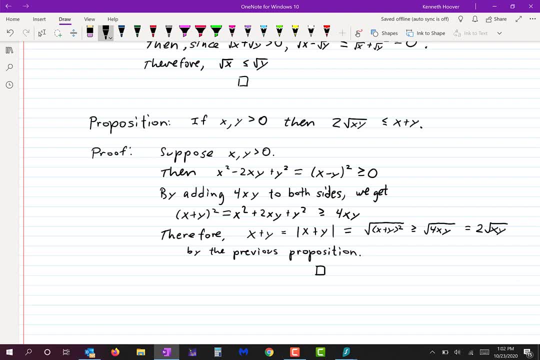 And I hope by now you're starting to get an idea of how direct proofs work.